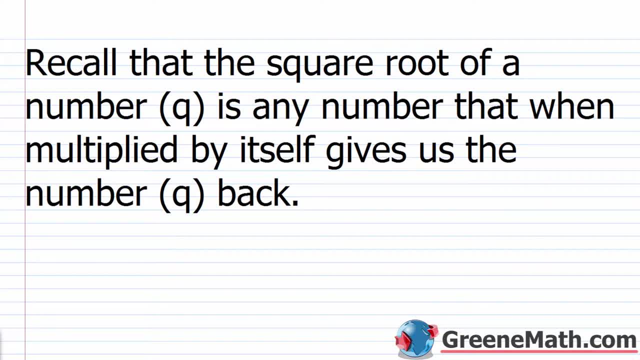 going to start out with the easiest scenario, which is where we deal with square roots. So I want you to recall that the square root of a number, and let's just say that number, is q, right, just as a placeholder for now. So this is any number that, when multiplied by itself, 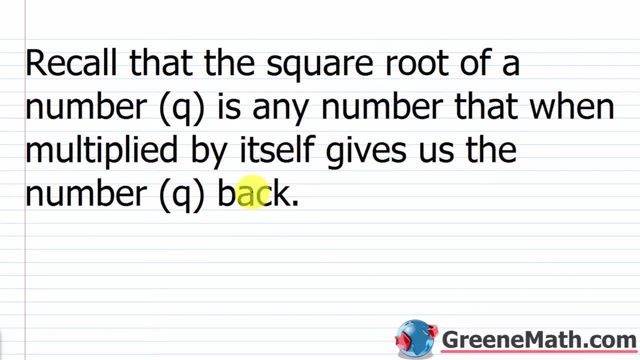 gives us the number q back. Now, by using a variable like q, a lot of you will stop and say that doesn't really make a whole lot of sense. So what you can do, you can just cross q out and you can just pick a number that you know is a perfect square. So, as an example, we know that. 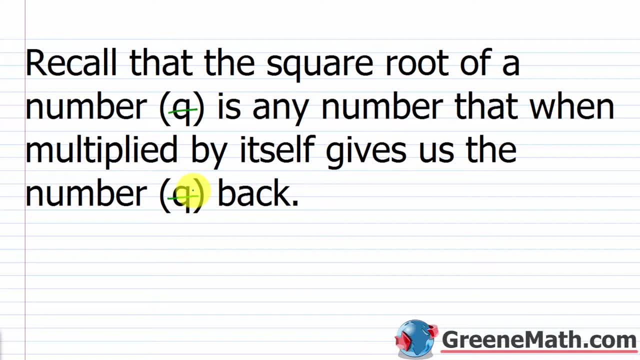 4 times 4 is 16.. So 16 is a perfect square. So we can say 16.. 16 and 16.. Now, if we reread it, we would say: recall that the square root of a number, 16 is any number that, when multiplied by itself, gives us the number 16. back Now we think about 16 as 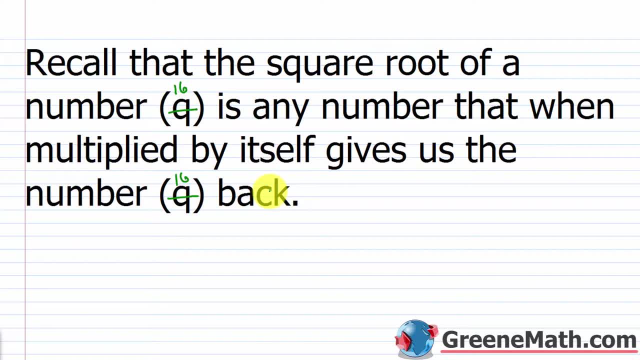 what Most of us would say. it's 2 to the fourth power. It's 2 times 2, which is 4.. 4 times 2 is 8 and 8 times 2 is 16.. We already know that 16 is 4 times 4, but we might forget that negative 4. 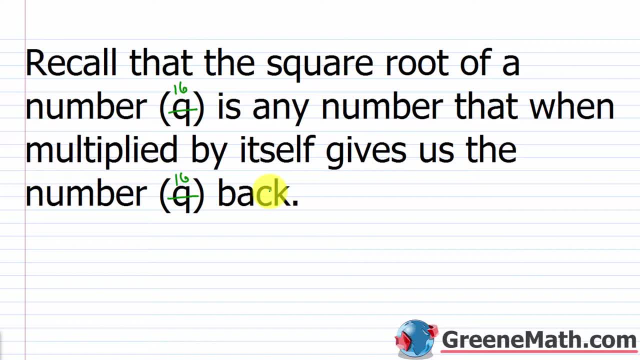 times negative. 4 is also 16.. So that's where this definition really comes in, where it says it's any number, So it could be more than 1.. So the square root of 16 would be 4, but also it would be negative 4.. Now, when we talk about square roots, we notate the positive square root, or what we 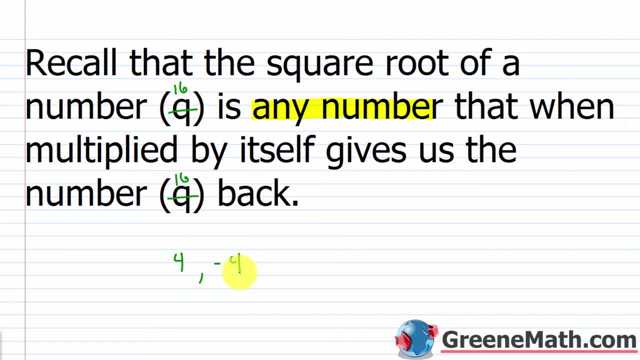 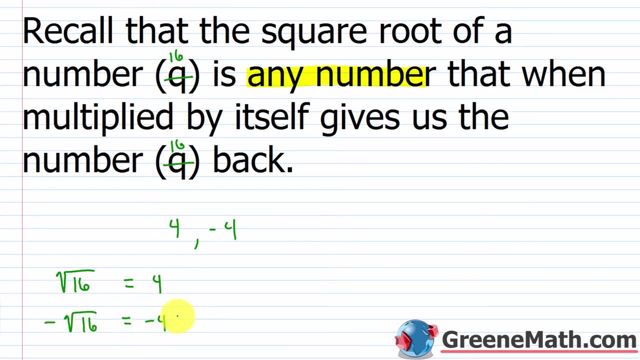 call the principal square root differently from the negative square root. So I would say the square root of 16 like this to ask for 4.. I would say the square root of 16 like this to ask for negative 4.. So this one right here is the positive, or we'd say the principal square root of 16.. 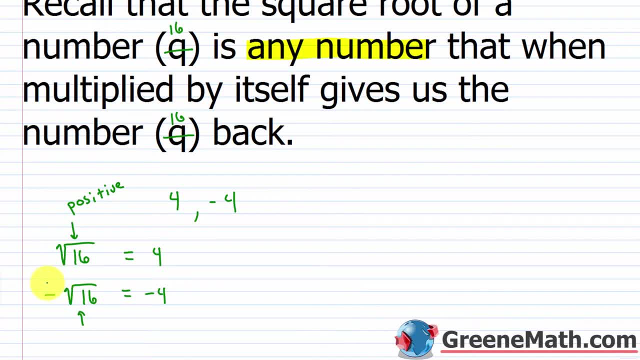 Whereas this guy right here- because we put that negative out in front- is asking for the negative square root of 16.. The difference between the two is just very, very slight. If I look at this one I say, okay, well, what positive number, when multiplied by itself, gives me 16.. Well, we know that off the top of our head, that 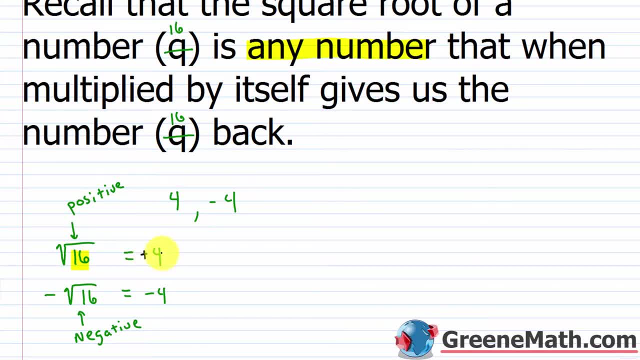 4, or more specifically, positive 4 times positive 4 would give me positive 16.. When I look at this one, I look at this negative out in front, I say, well, what negative number, when multiplied by itself, would give me 16.. Well, negative 4 times negative 4 would be 16.. So I would say that's. 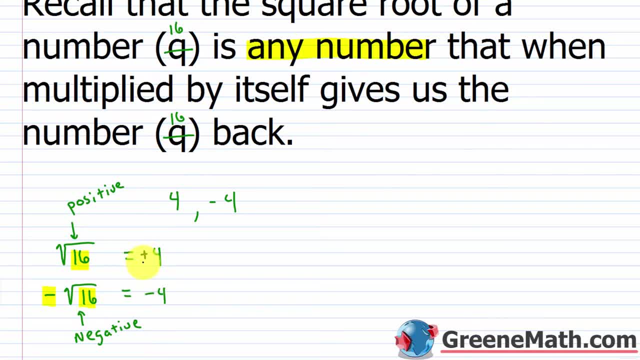 16.. So those are the two different notations that you'll run across. If you see something like what is the square root of 25.. This is just asking for the principal square root, so they just want 5 back. If you see what is the negative square root of 25, like that they're asking for: 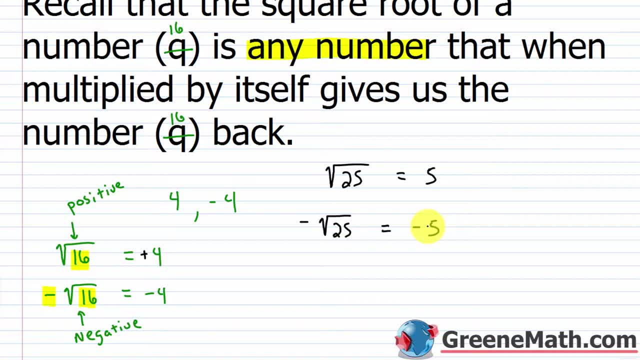 negative 5.. As we learned back in algebra 1 when we started looking at the quadratic formula, there's a shortcut notation for this. I don't need to separate these two like this. I can just put plus or minus like this in a compact form and then put square root of 25.. This is asking for the 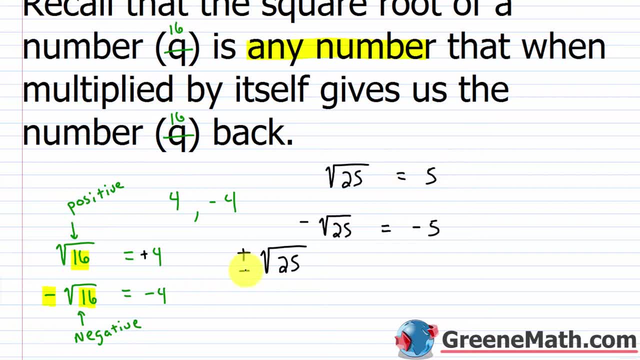 positive or principal square root of 25.. It's also asking for the negative square root of 25.. So this I can put is equal to plus or minus 5.. So I'm accounting for both possibilities. The positive square root of 25 is 5.. The negative square root of 25 is negative 5.. So this is again just a more. 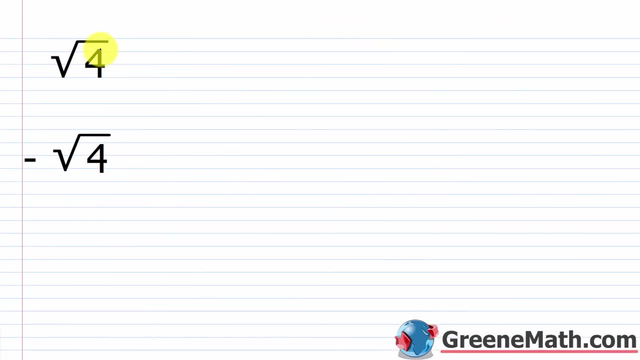 compact way to do it. So I'm going to put plus or minus like this in a compact form and then put square root of 25 to write things. So let's just look at a quick example here. So we have the principal square root of 4.. So that's asking for what positive number when multiplied by itself. 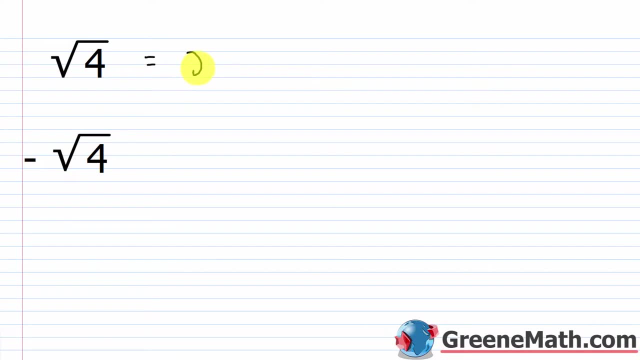 would give me 4.. All of us know that would be 2.. 2 times 2 is 4.. Now with this one we have the negative square root of 4.. So we're saying, hey, what negative number when multiplied by itself. 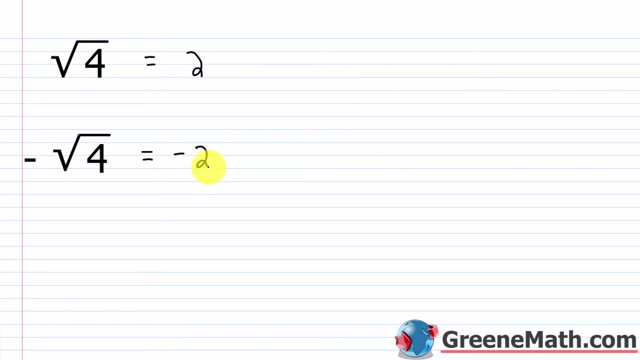 would give me 4 and that's negative 2.. Now again, if you want to practice that more compact notation, you could say plus or minus 5.. So that's asking for what positive number, when multiplied by itself, would give me 4.. So that's asking for what positive number when multiplied by itself. 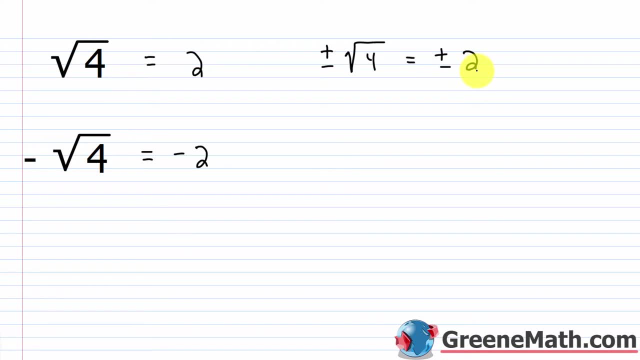 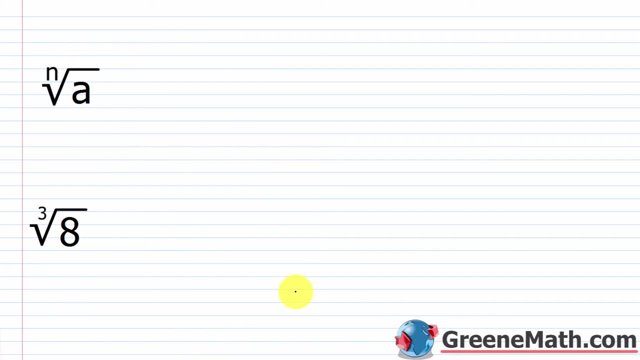 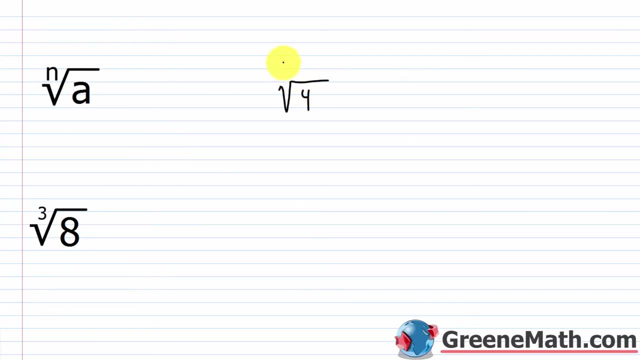 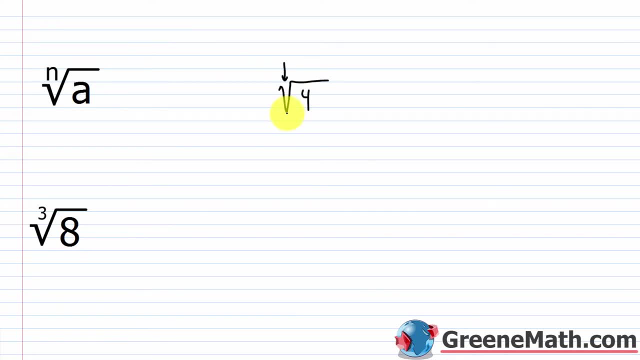 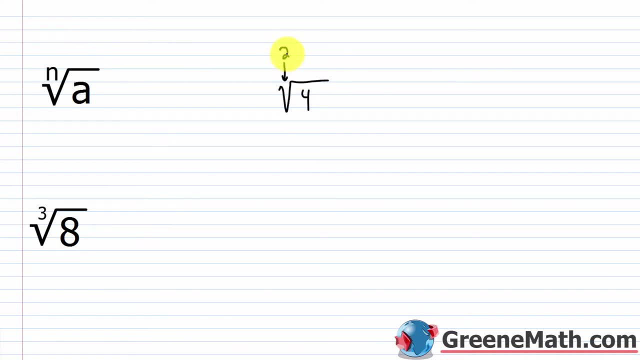 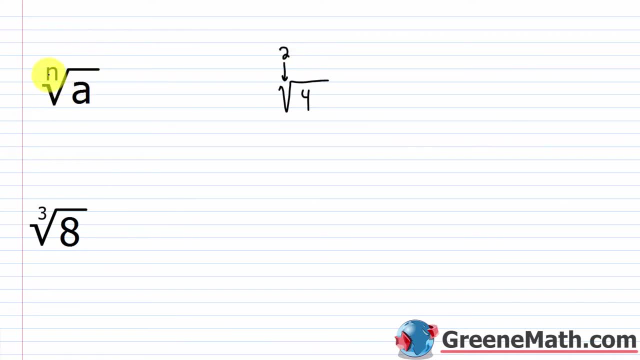 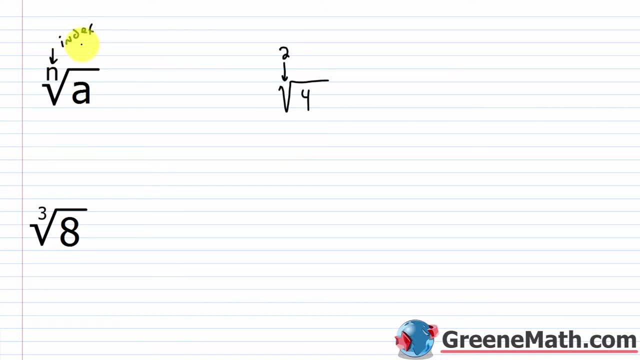 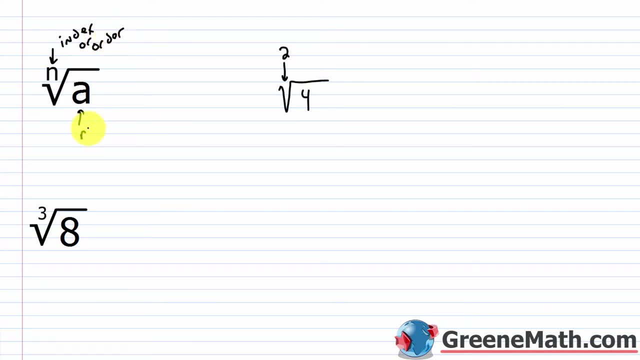 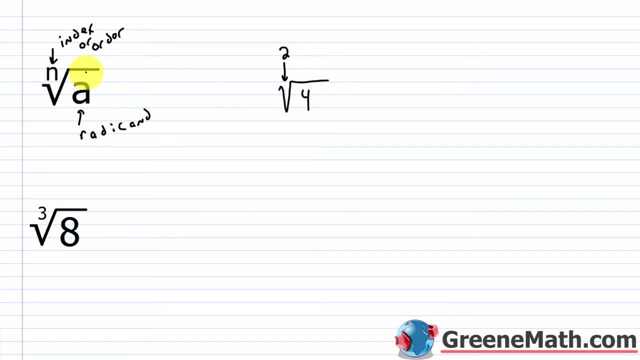 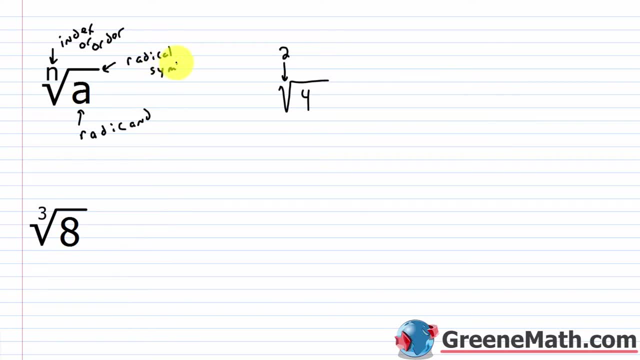 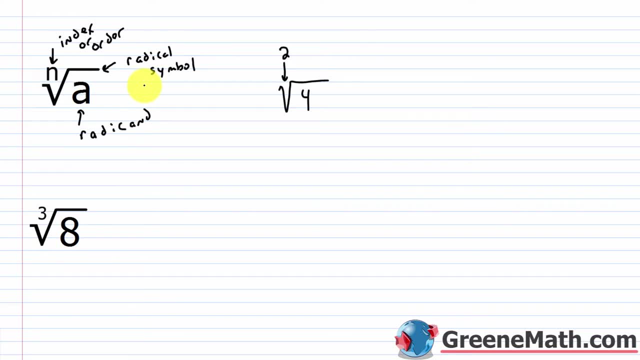 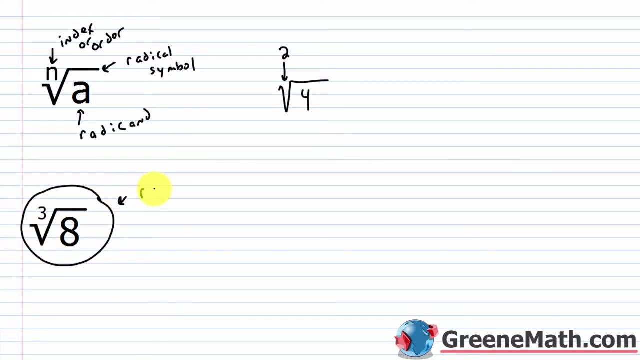 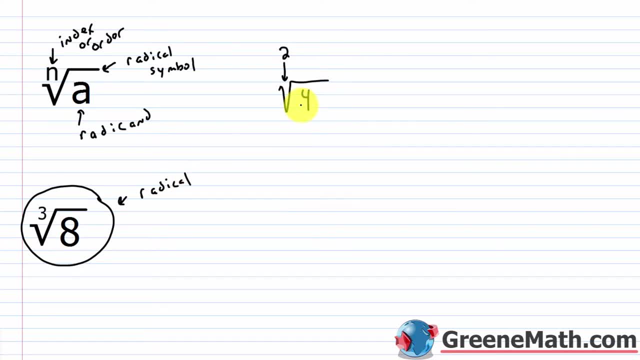 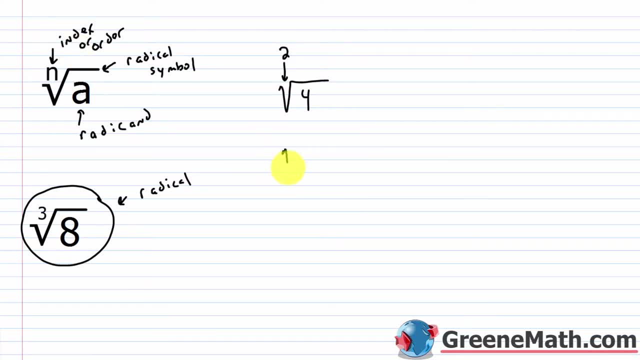 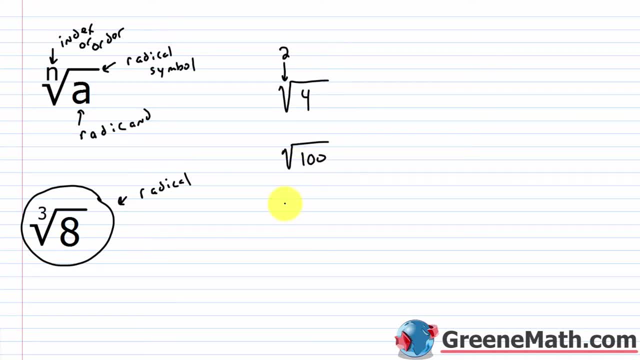 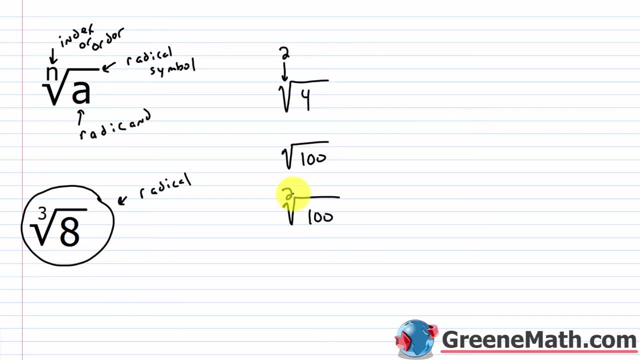 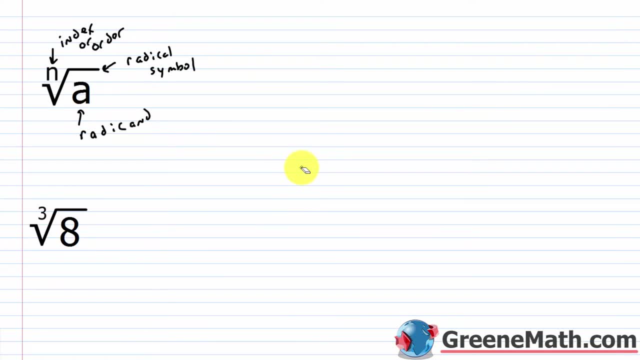 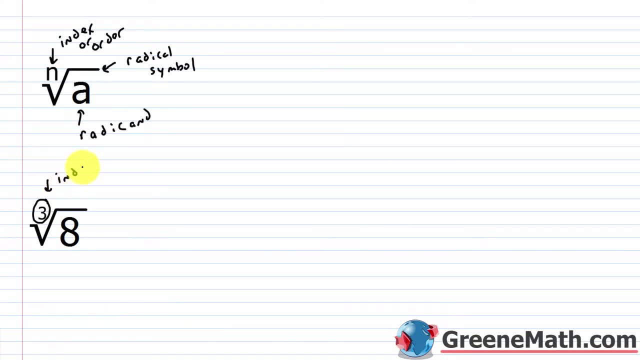 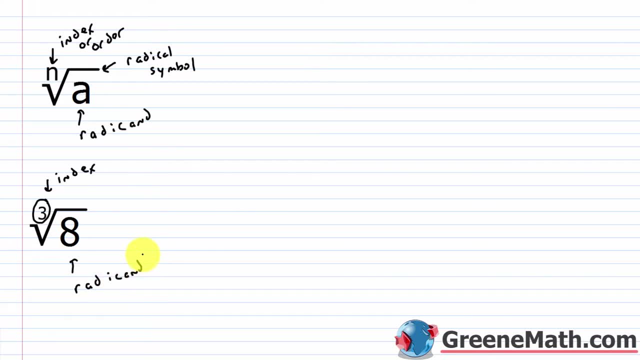 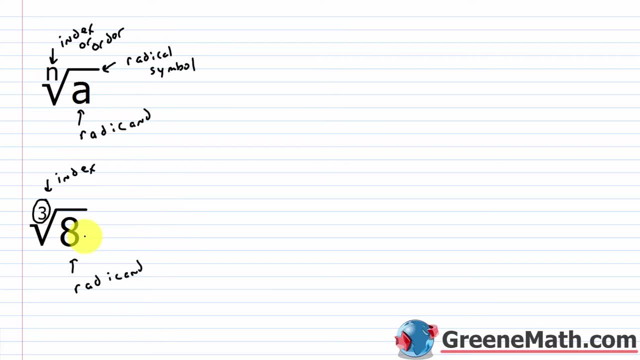 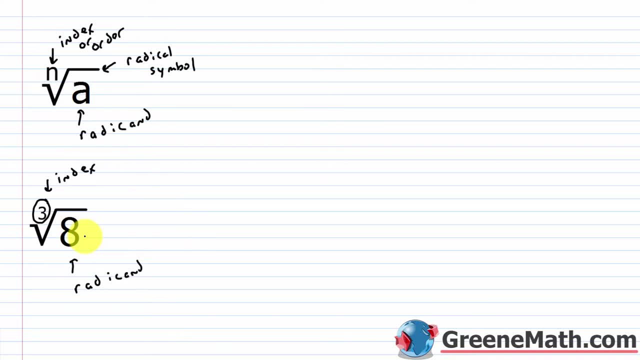 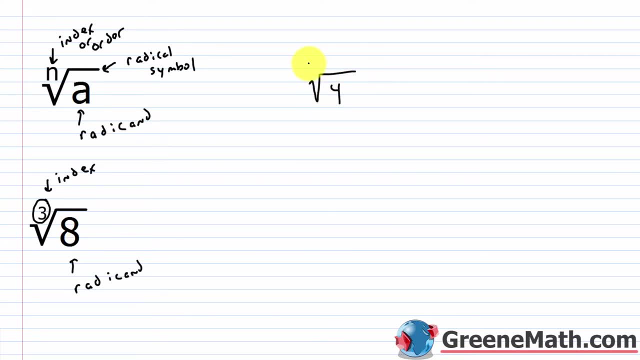 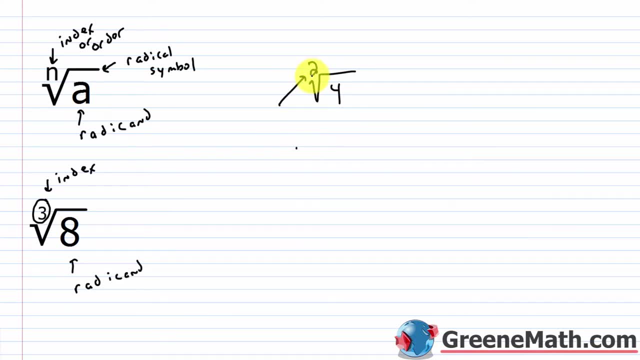 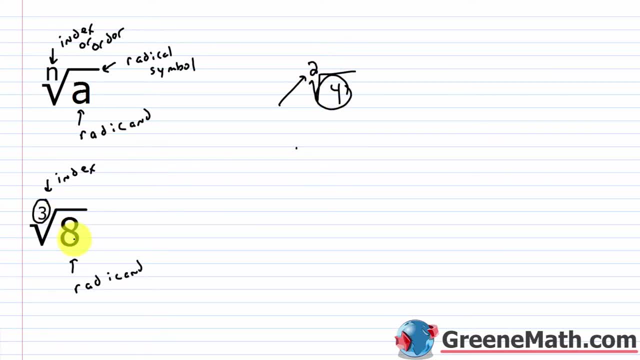 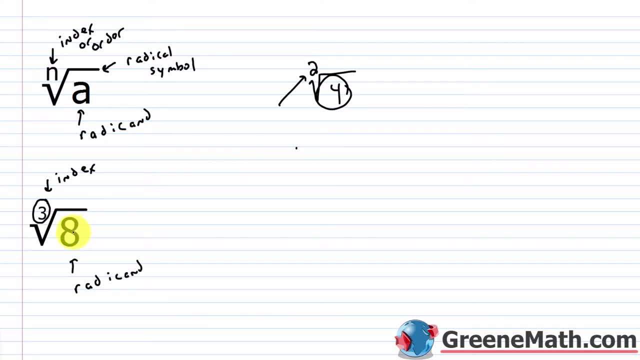 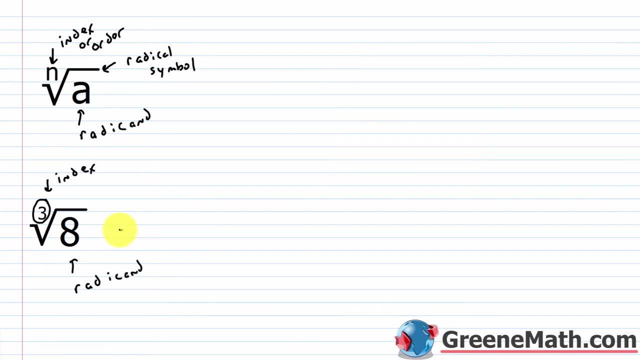 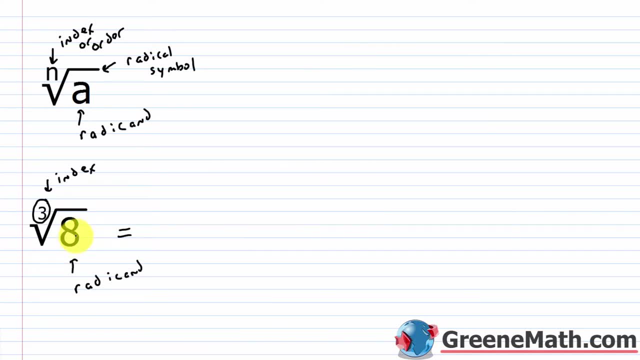 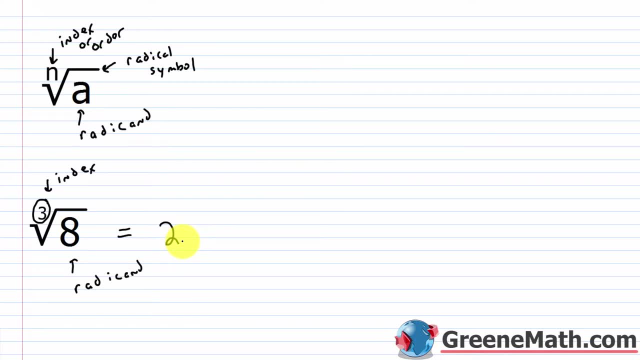 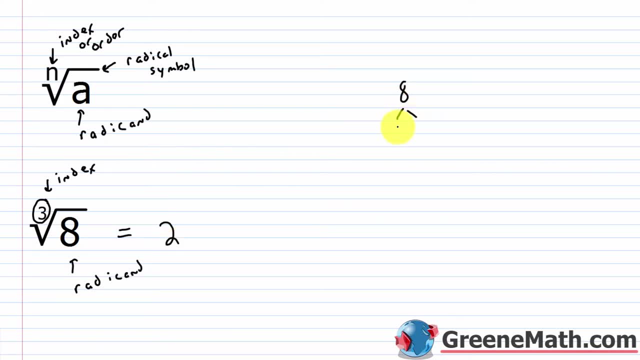 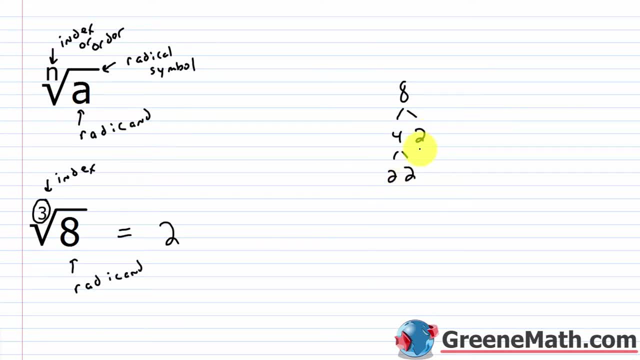 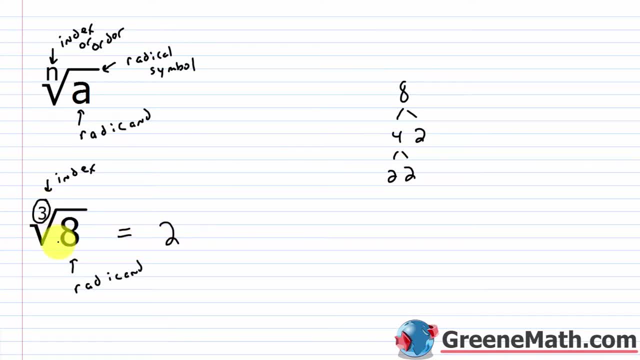 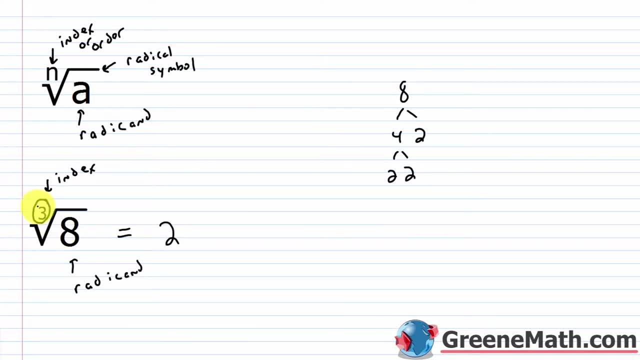 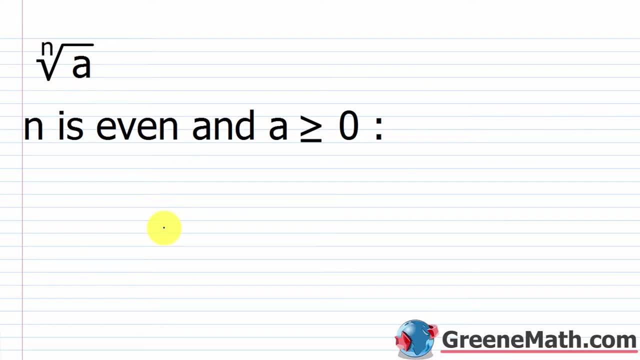 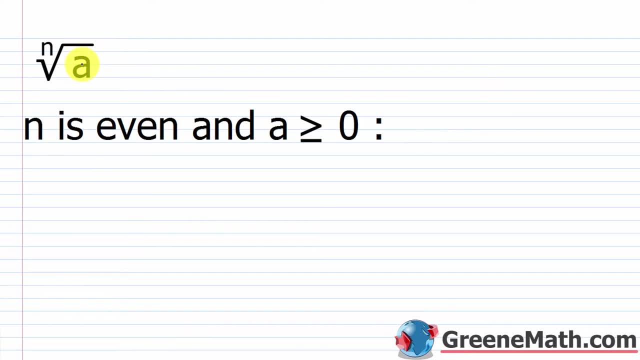 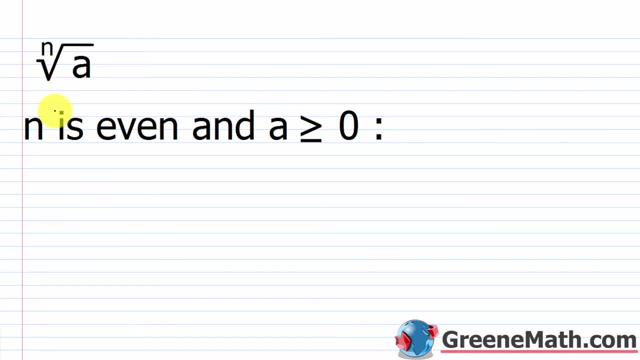 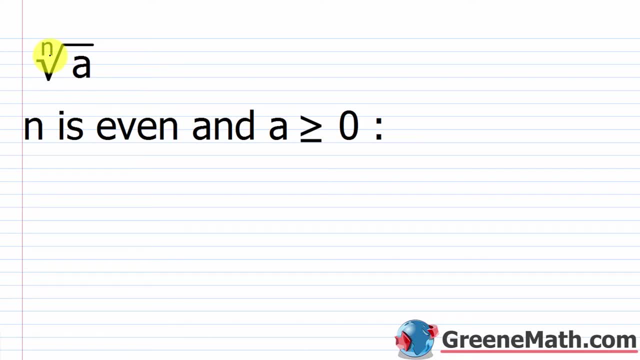 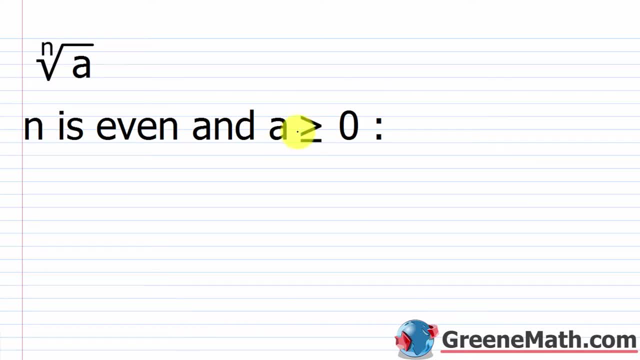 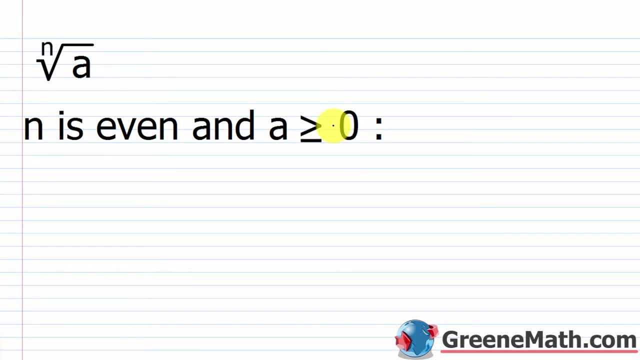 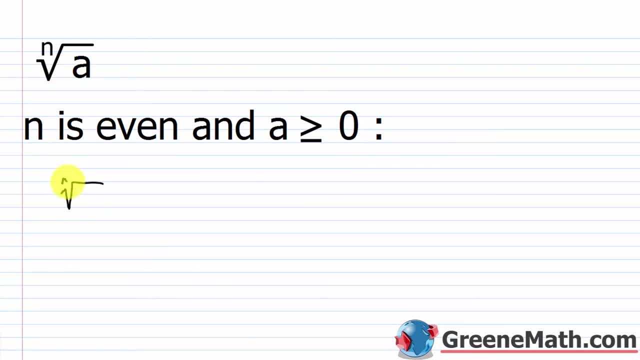 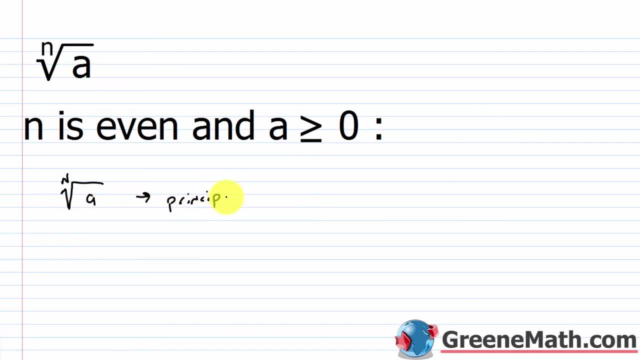 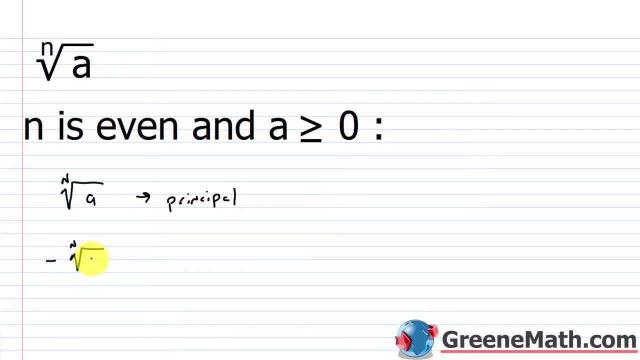 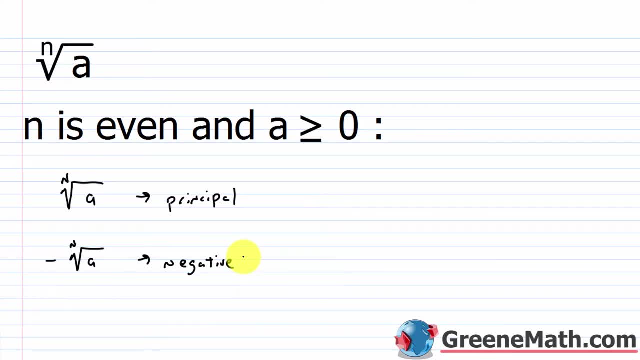 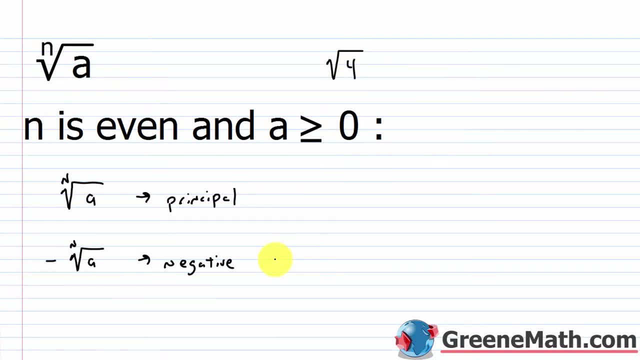 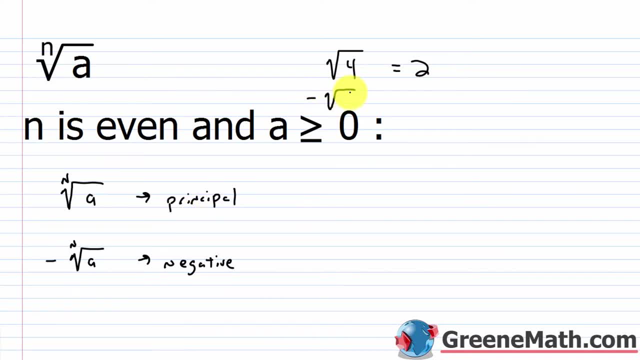 would give me 4.. So that's asking for what positive number, when multiplied by itself, would give me 4.. So that's asking for what positive number, when multiplied by itself, which is negative: 2. But again, it's not just with a square root, it could be a fourth root. 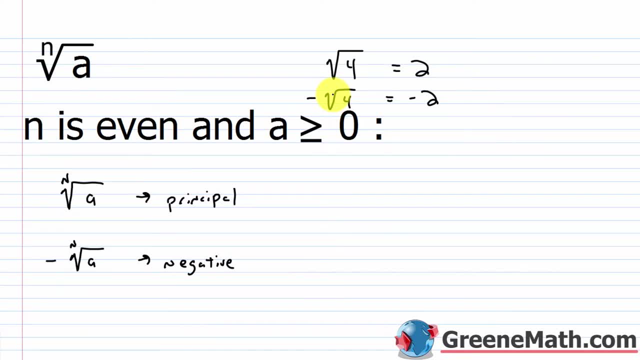 or an eighth root, Something easy to do. let's say we had the fourth root of 16.. So the fourth root of 16,. many of you know that 2 to the fourth power is 16.. 2 times 2 is 4,. 4 times 2 is 8,. 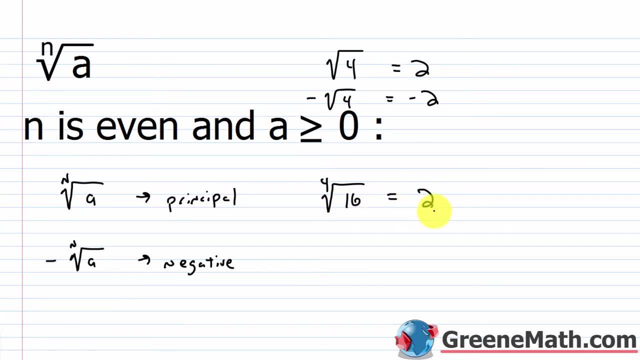 8 times 2 is 16.. So we know this would be 2.. But then you'd also have to account for the negative fourth root of 16. This would just be negative 2.. And if I multiply negative 2 by itself four times, 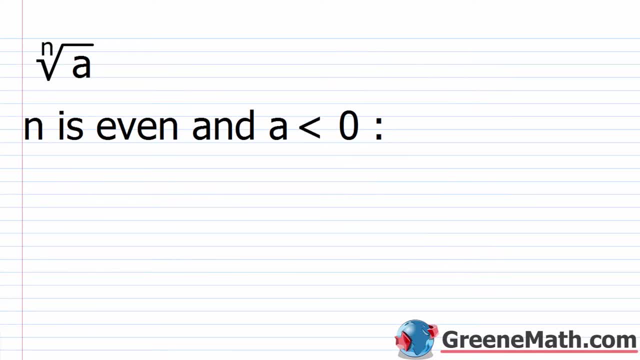 I would get positive 16 as a result. All right, the next scenario I want to talk about: if we have the nth root of a and n is even and a is less than 0. So now a is a negative value. 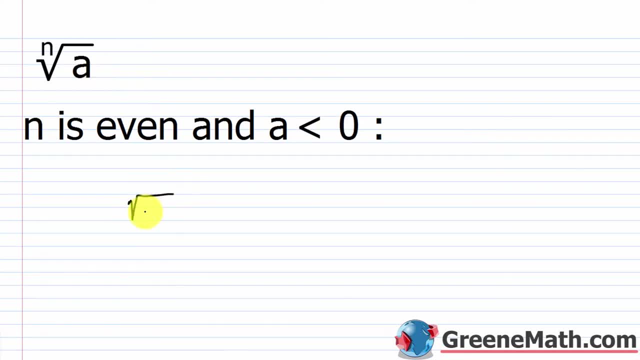 So you'll recall this from Algebra 1, where we said we had the square root of I don't know, let's say negative 16.. What happens here? Well, it's not a root, real number, And we're going to learn how to deal with this in Algebra 2.. We didn't talk about it. 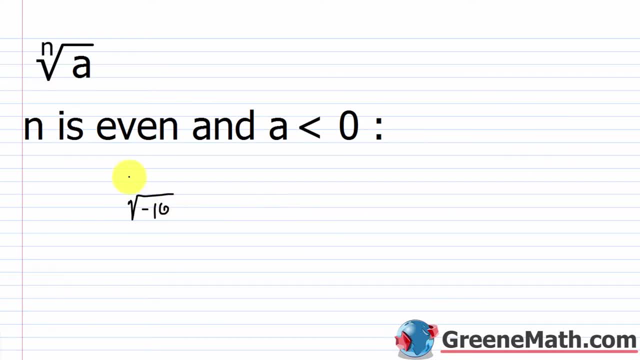 in Algebra 1,. but we will have a way to evaluate this using something known as imaginary numbers. But we haven't gotten to that yet. So for right now, we just say that this is not real, This is not a real number. So again, if n is even so, 2,, 4,, 6,, 8,, 10,, 12,, whatever it is. 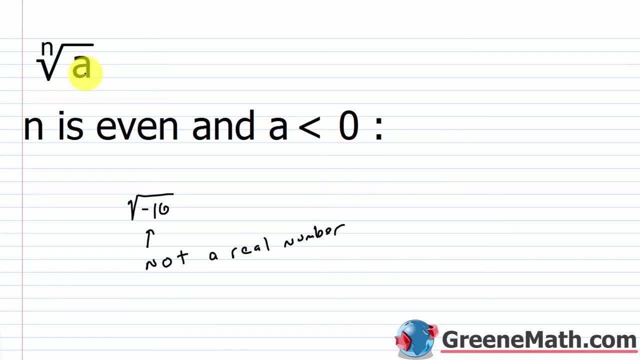 and a is less than 0,, a is a negative value, then you're going to write that it's not a real number. So let's say you had the fourth root of, let's say, negative 625.. Again, this is, even this is negative, so it's not a real number. 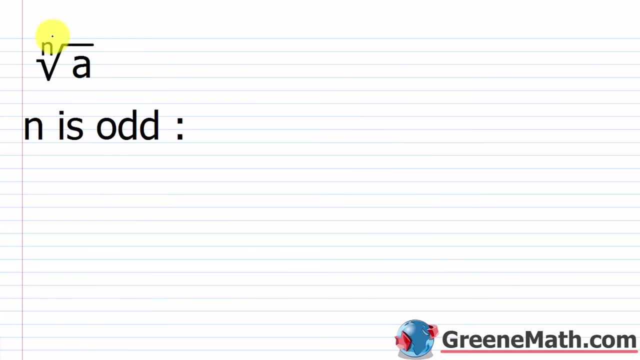 All right. the final scenario: if you have n, that's odd, okay, so your index is odd. a can be whatever. It can be positive, it can be negative, it can be negative. So if you have n, that's odd, okay, so your index is odd. 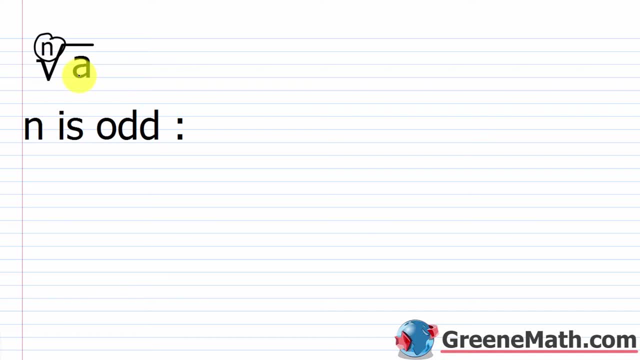 it can be whatever. It can be positive, it can be negative. So if you have n, that's odd. it can be negative, it can be 0, it can be whatever you want it to be. You're only going to have one root, And the reason for this deals with the rules for positives and negatives. 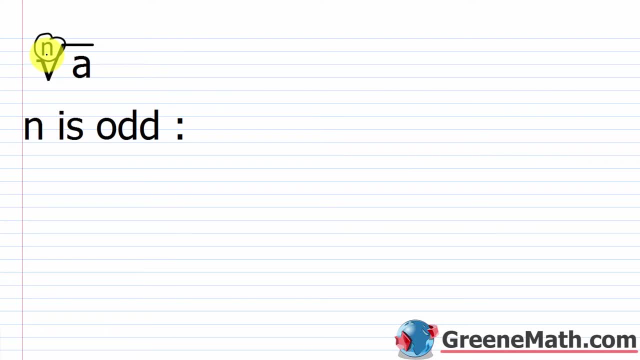 If I multiply a negative by itself an odd number of times, I get a negative. So if I had something like, let's say, the cube root of negative 8.. So what number, when multiplied by itself three times, gives me negative 8?? Well, that's negative 2.. Negative 2 times negative 2 is 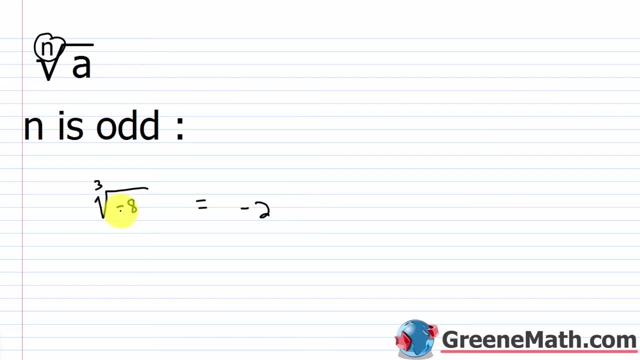 positive 4.. Then positive 4 times negative. 2 is negative 8.. Just keep in mind that you are allowed to have a negative radicand. if this guy is odd, okay, It's just the case where you can't have a. 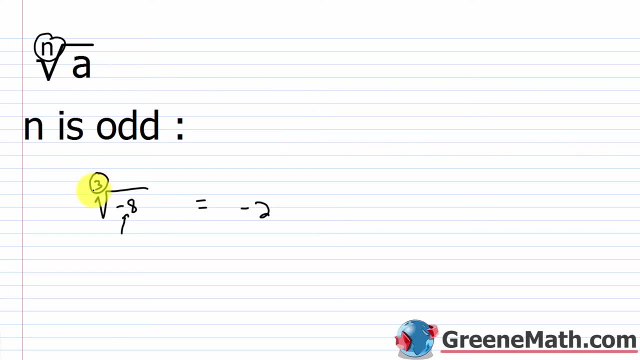 negative radicand, when that guy is even So a lot to kind of throw at you, especially if you didn't learn this back in Algebra 1.. It's just one of those things where you just have to practice enough and it's something you're going to have down pretty much right away. All right, so let's. 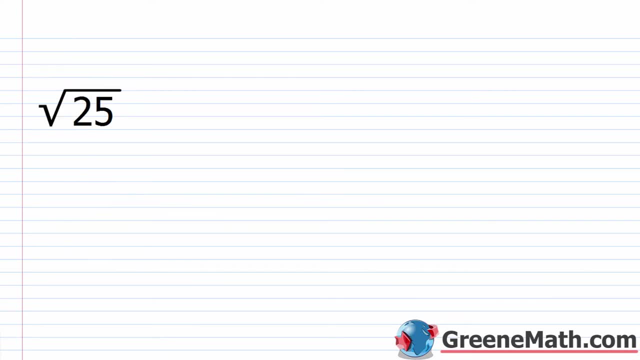 just take a look at some really easy examples. So we've seen this already. If I had the principal square root of n, I would have a negative radicand. If I had a negative radicand, I would have a 25.. We know, that would be what I'm just asking for: a positive number that, when multiplied by 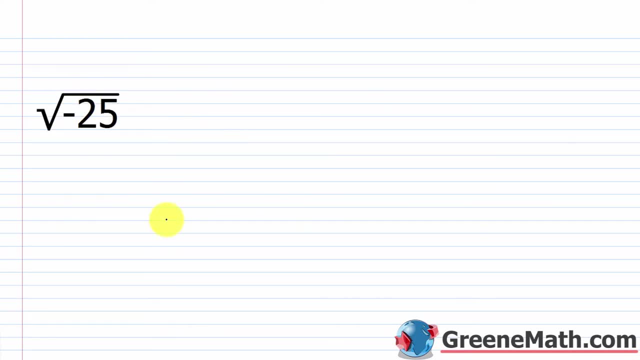 itself gives me 25.. We know that would be 5.. Then what about the square root of negative 25?? Now again, if I have a negative radicand and I have an index, that's even in this case. 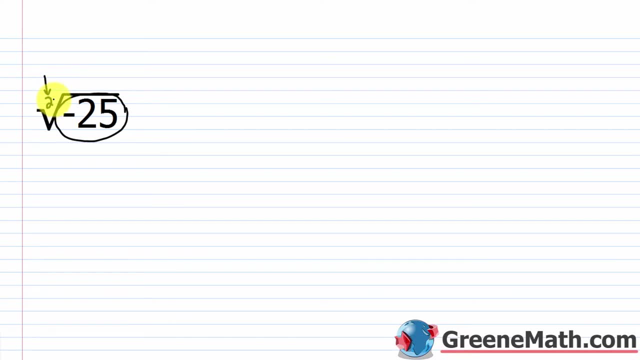 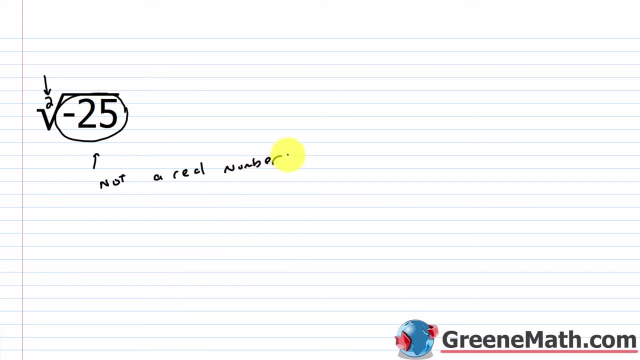 not a real number. Now, don't get this confused with what we're going to see now. Here we have the negative square root of 25.. Underneath the radical symbol, I have a positive value. So I'm okay, This is positive. It's the negative outside that's telling me: hey, I want the negative. 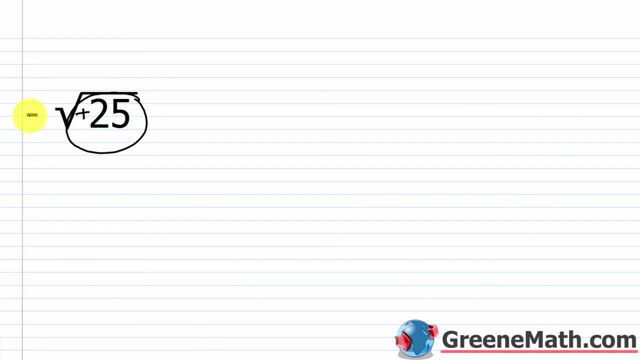 square root of 25.. That's a big source of confusion, So make sure you understand the difference between the two. The negative square root of 25 is just asking for what negative number, when multiplied by itself, will give me 25, and that's negative 5.. Negative 5 times negative 5 is 25.. 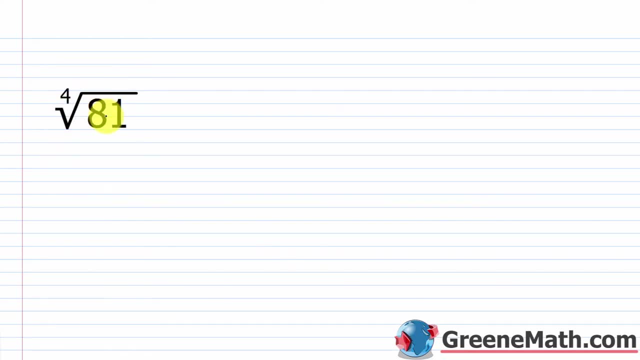 For the next example, we have the principal fourth root of 81. So we're asking for what positive number, when multiplied by itself four times, is going to give us 81. Well, some of you will know right away, that's 3.. If you didn't again, you can use a factor tree. 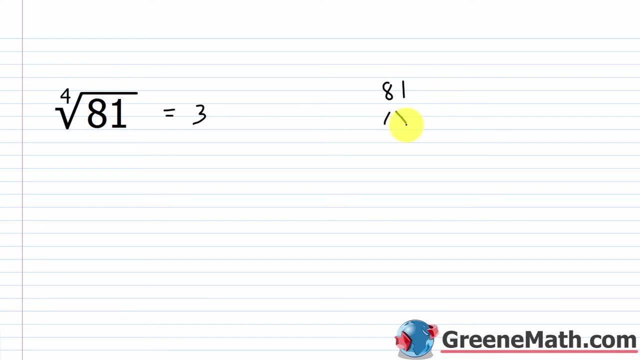 So take 81. And break it down. Most of you will know that 81 is what It's 9 times 9.. 9 is 3 times 3.. So just a quick factor tree will show you: 3 times 3 times 3 times 3, or 3 to the fourth, power is 81. So that. 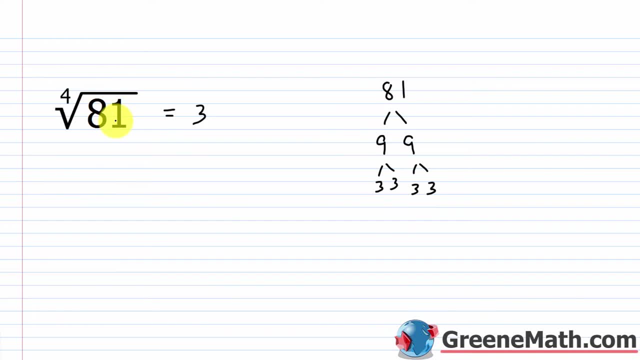 means, if I'm looking for a positive value now, when multiplied by itself four times, it's going to give me 81. We know that's going to be 3.. All right, what about the cube root of negative 64?? Because this index is: 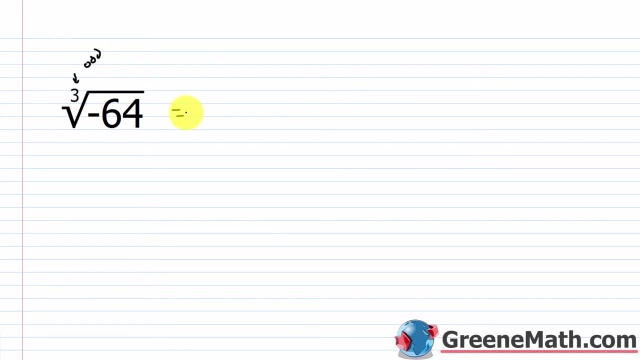 odd. I know I'm going to have one answer and I know that the negative is allowed. This is okay Again, because this is an odd index: A negative times, another negative times, another negative or three negatives or an odd number of negatives in general will produce a negative. So all you. 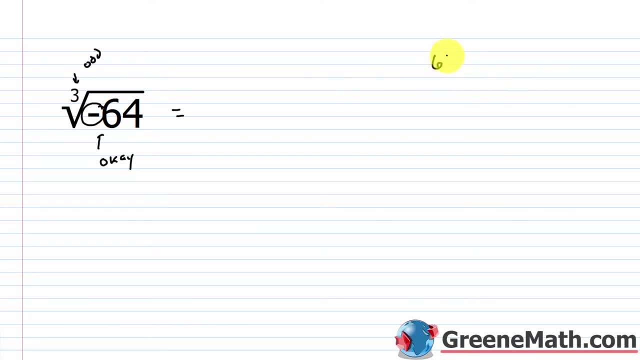 got to ask yourself is: take 64.. Forget about the negative for a second. 64 factors into what It's 4 times 16.. 16, is 4 times 4.. So without going into 4 as 2 times 2,, I know I have 4 times 4 times 4, or 4 cubed. 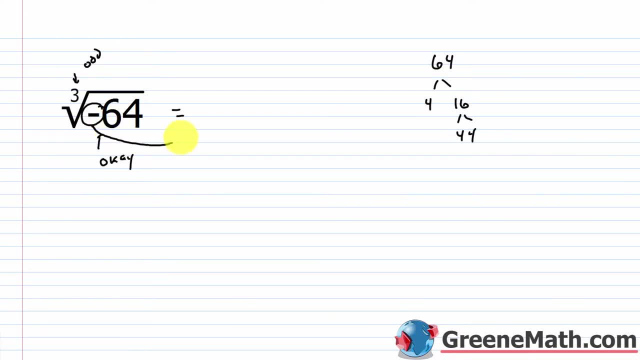 That gives me 64. All I got to do is just drag this negative over here and say this is negative 4.. Because the negative times, the negative times, the negative will give me a negative back. So negative 4 times itself, three times, will give me negative 64.. All right for the next one. 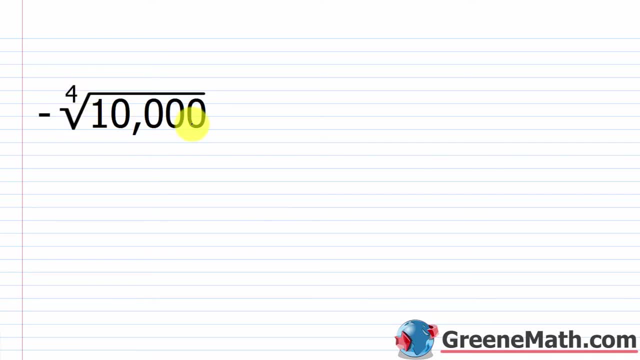 we have the negative fourth root of 10,000. So what are we looking for? We're looking for a negative number that, when multiplied by itself four times, is going to give us 10,000. Now, so I'm just going to put a negative out in front because I could just forget about it. 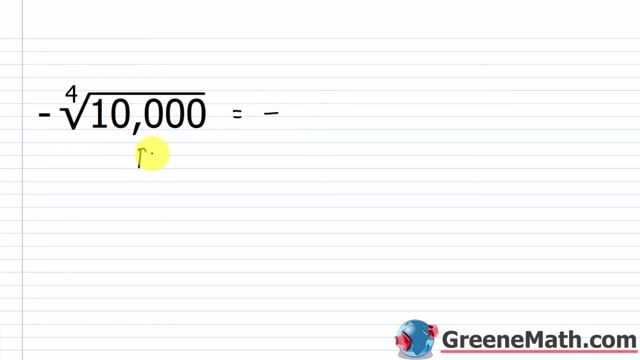 now. Now I just think about 10,000.. 10,000 is a power of 10, so it's really easy, right? It's a 1, followed by 1, 2, 3, 4 zeros. So that means it's 10 to the fourth power. So the way I get that is: 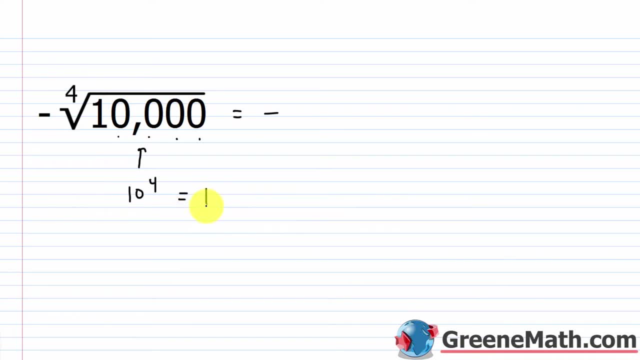 if I'm evaluating something like this, 10 to the fourth power, you write a 1, and you follow it by zero. So this is 1, 2,, 3, 4.. So kind of a cool trick, if you don't know that, So I automatically. 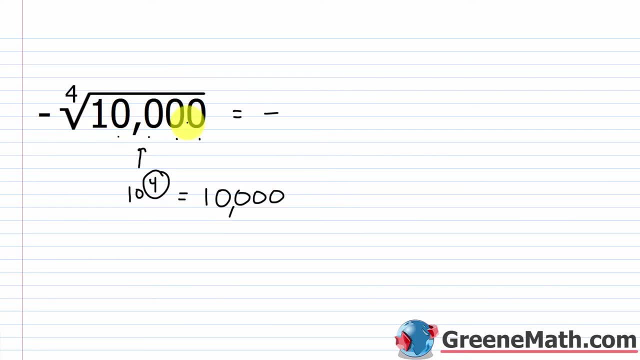 know that if 10 to the fourth power is 10,000, the fourth root of 10,000, forget about the fact that it's the negative fourth root. We've already accounted for that. The fourth root of 10,000. 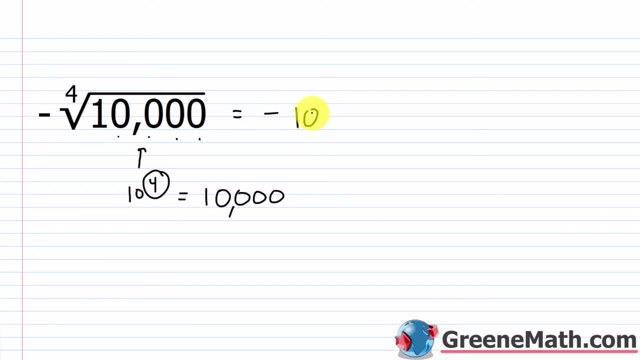 would just be 10.. So we just put negative 10 here as our answer, right. Negative 10 times negative 10 is 100.. 100 times negative 10 is negative 1,000.. Negative 1,000 times negative 10 is 10,000.. 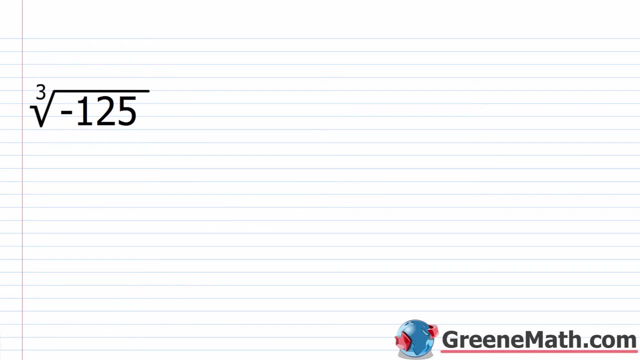 All right, let's take a look at another one. Let's say you saw the cube root of negative 125.. So again, if I'm thinking about something like this, this is negative. Three negatives makes a negative. So I just start out with putting a. 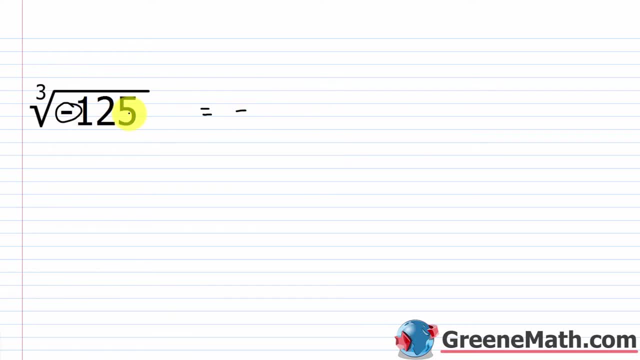 negative there, Then you can just forget about it and you can say, okay, well, 125.. 125 would factor into what? 25 times 5.. 25 is 5 times 5.. So 5 cubed would be 125.. So what I'm looking for here. 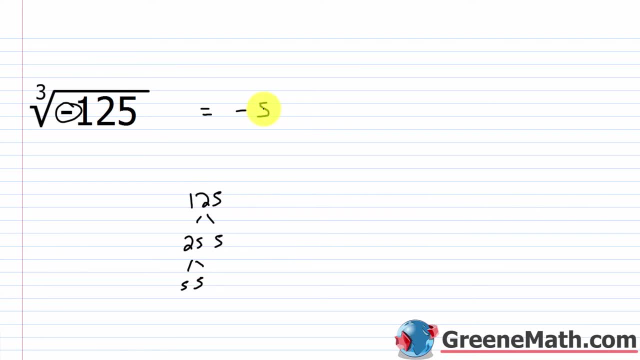 is negative 5.. Negative 5 times negative 5 is 25.. 25 times negative 5 is negative 125.. All right, last one. We have the principal fourth root of negative 16.. So again, I have a negative radicand and I have an even index. So when that happens, 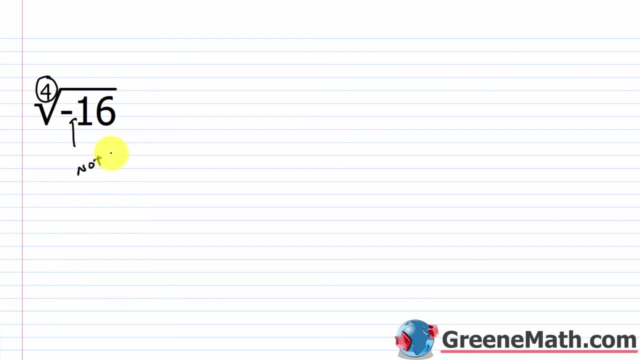 we don't have a real number. This is not a real number And again, the reason for that is I can't take a negative and multiply it by itself four times and end up with a negative. All right, it's going to give me a positive. An even number of negatives will always give me a. 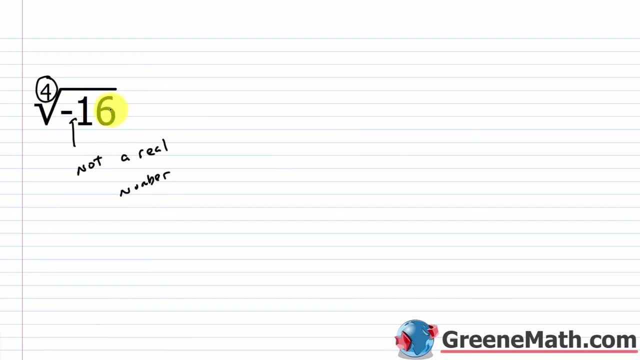 positive, And so that's why this value doesn't exist using real numbers. Well, let's take a look at another rule. that's pretty time-saving for us If we have the nth root of a to the nth power, so something like if you had the fourth root of, let's say, 2 to the fourth power. 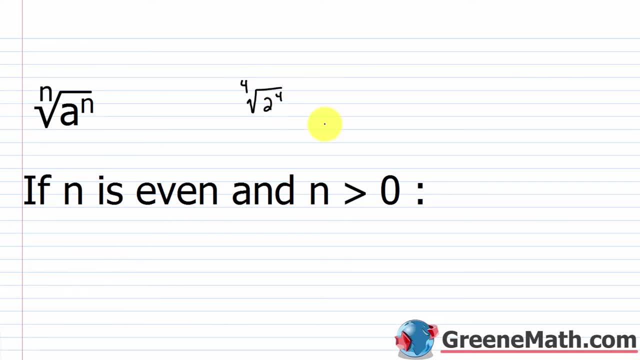 what would you guess would happen there? Well, you know from your studies of Algebra 1 or 2, hopefully you remember- that this ends up canceling with this and you're left with this right. So if n is even so, in other words, if this is even and this is even, they're the same value. 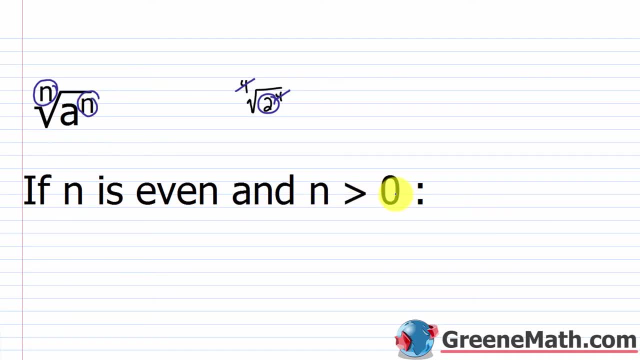 and n is greater than 0, so even and greater than 0,. then what we're going to find is we have the nth root of a. to the n, We'll say: this is equal to the absolute value of a. So, as an example, 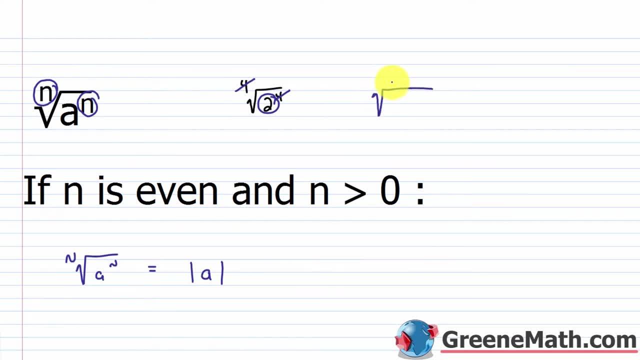 let's just say we took something like 5.. So we take the 6th root of 5 to the 6th power. Now you don't even need to calculate what 5 to the 6th power is, You can just say: okay, well, if I took 5 and I raised it to the 6th power. 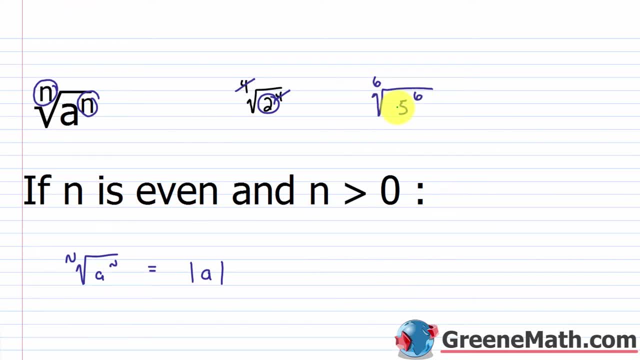 whatever number that is, once I take the 6th root of it, I'm going to be right back to 5.. So this will cancel with this and I'm left with this. So this would be equal to 5.. As another example, 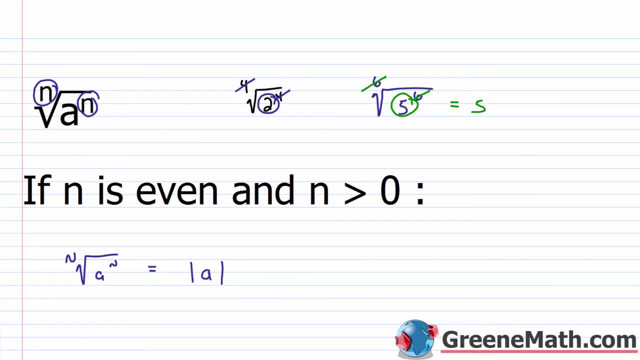 let's say I was working with a negative And to make it real simple, let's just make it negative 2.. So if I had the square root of negative 2 squared, what would that be equal to? Well, some of you might say. 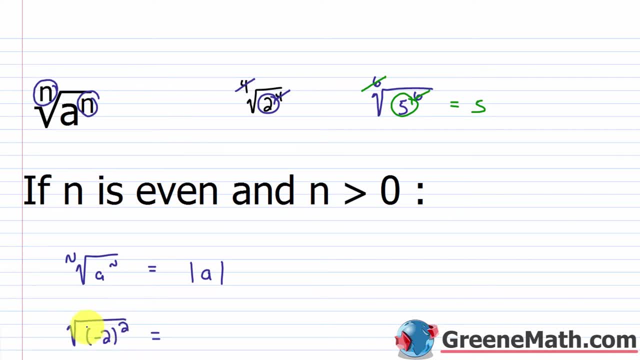 oh, that's not a real number. You have a negative down there. Well, think about squaring this first. If I did negative 2 squared first, that would give me 4.. And if I took the square root of 4,? 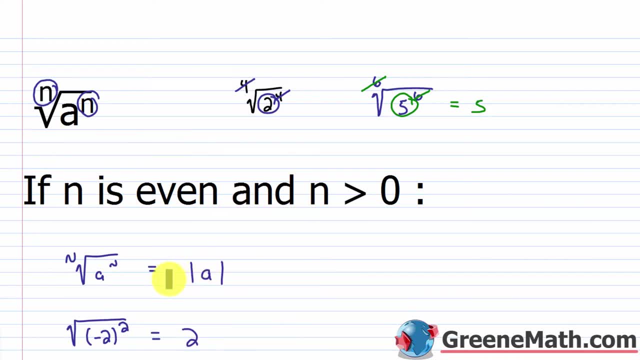 I would get 2.. So that's where this definition comes into play. Notice how we say it's the absolute value of a. So if we're saying a here is negative 2, well, the absolute value of negative 2 is 2.. And that comes from that again, that squaring. 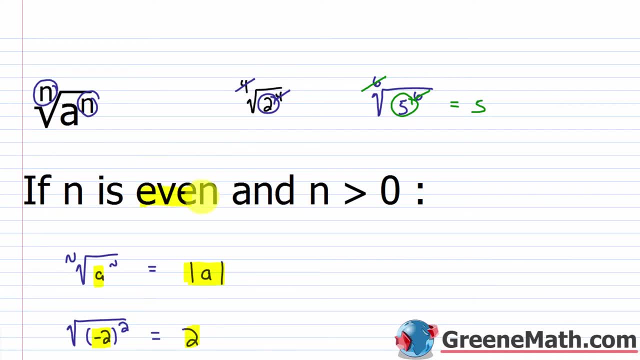 operation- Or in this case it could be anything, that's even So. it raises them to the 4th power, the 6th power, the 8th power, the 10th power. Whatever, it is an even number of negatives. 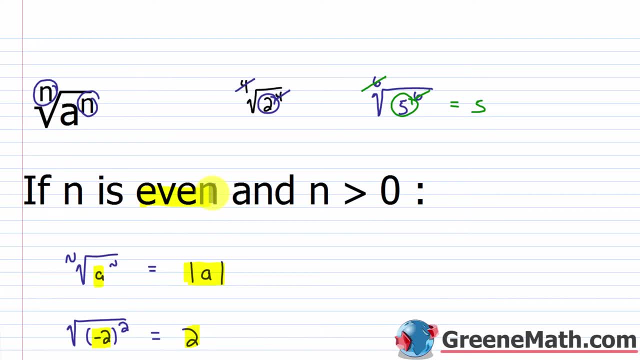 will give us a positive value. Then when we perform that root operation, we're going to go back to the absolute value of whatever. that was right, Because we took a positive, took the root of it and we went back to whatever the absolute value of that was. 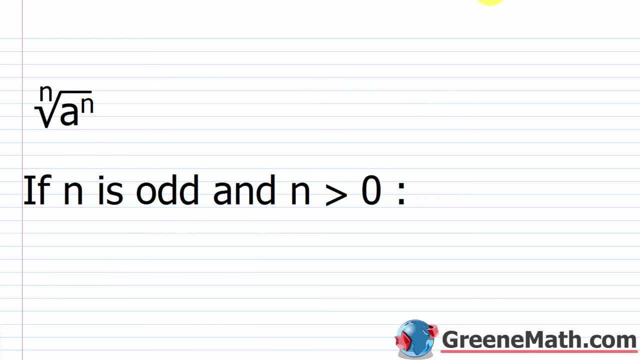 All right. the next one we want to talk about is the other scenario, where n is odd. So if n is odd and n is greater than 0, then what's going to happen in this case? So this is odd and it's greater than 0. In this particular scenario, these two will just cancel each other. 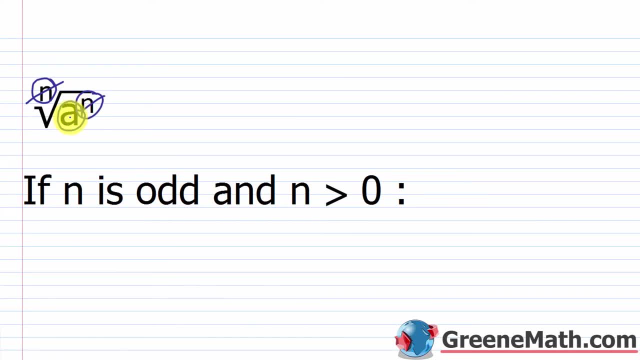 out and you're just left with a. So the only difference is, when you have an even involved, you got to say, in case you're a, in case this radicand was negative, you've got to account for that. So you've got to account for that. 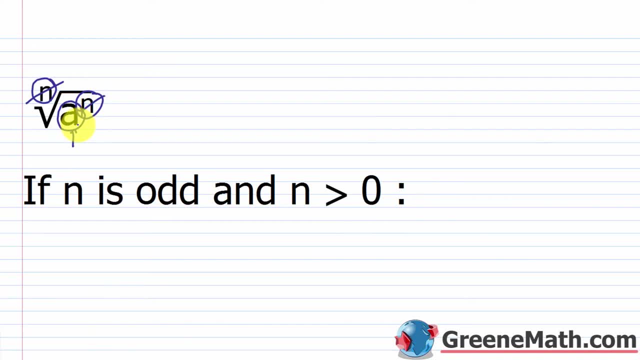 You've got to account for the possibility that you do an even number of factors of that guy right, Because you're raising it to an even power. It's going to end up being a positive. Then you take the root and knocks it back down to the absolute value of that. 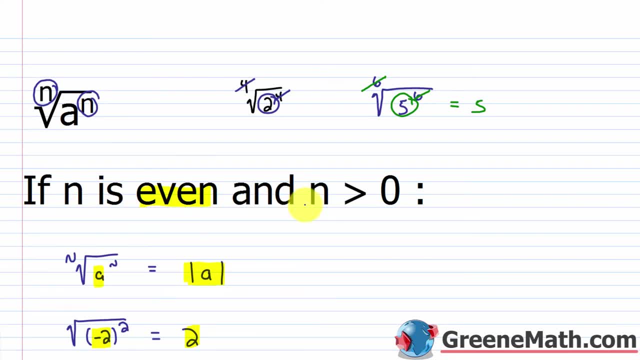 So that's all we're saying here. Again, n is even and n is greater than 0.. All we're saying is, if this guy was negative, an even number of negatives would have made it positive. So you get back to the absolute value of that In this scenario, because n is odd. 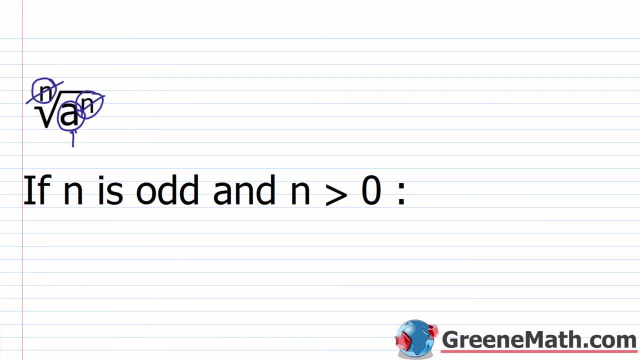 an odd number of negative factors would give you a negative. it's okay. So, as an example, let's say I had the cubed root of I don't know, negative 2 cubed. Well, this is just going to be. 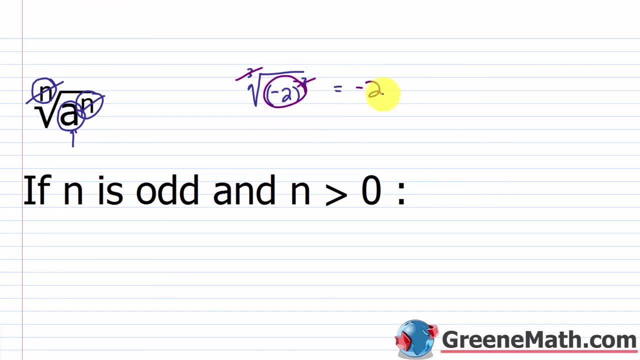 what This would cancel with this, and I just have negative 2.. All right, so let's say we saw something like the sixth root of negative 7 to the sixth power. So, again, without even going through and saying, okay, well, negative 7 times negative 7, without giving you six factors of 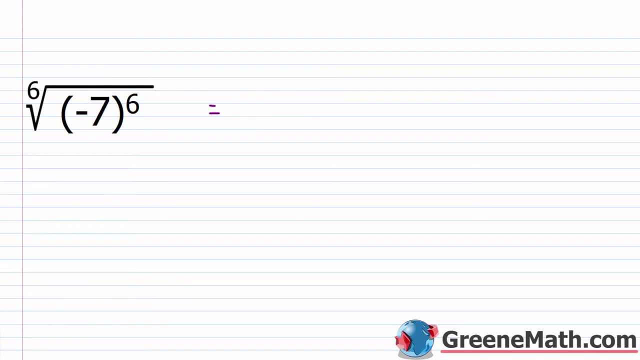 negative 7, you're going to get a negative 2.. So you're going to get a negative 2.. So you're going to, and then taking the sixth root of that, you automatically know that this would cancel with this, but I'm not left with negative 7.. I'm left with the absolute value of negative 7, which is: 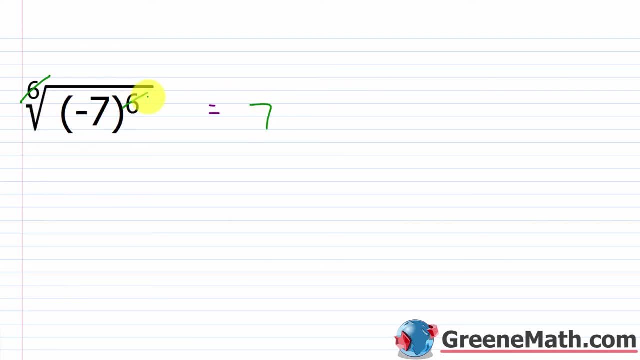 7, right. So it's a little bit more complicated than just canceling things. I don't want you to make the mistake of just canceling things and saying, okay, this is negative 7, because that would be wrong. Taking negative 7 to the power of 6 would have made it positive, and then taking 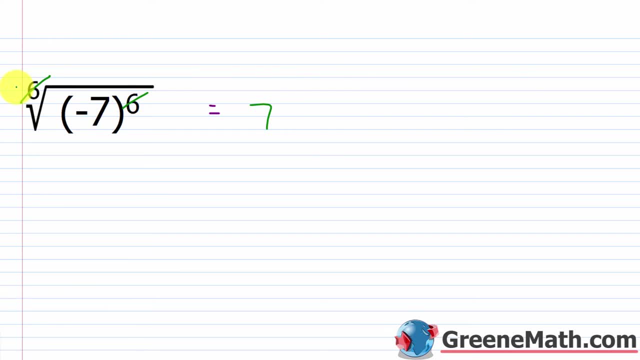 the sixth root of that would have brought you back to positive 7.. So it's important to realize that this is equal to the absolute value of negative 7, which is 7.. So here's an example where we have an odd index. So we have the cube root of negative 9 cubed. So in this case you can just kind of 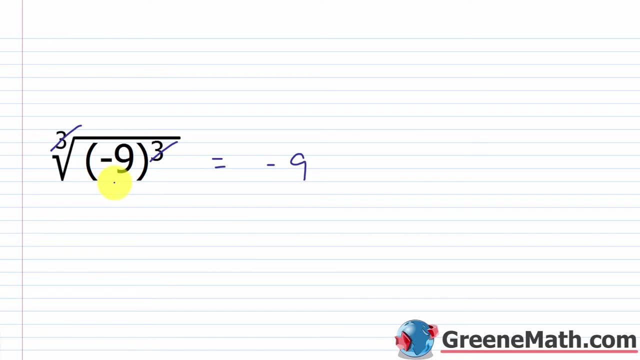 cancel these and say I'm just left with negative 9, right? Negative 9 to the third power would still give you a negative result, right? So when I take the cube root of that, it would still be a negative. So I'm going to take the cube root of that and I'm going to take the cube root of that. 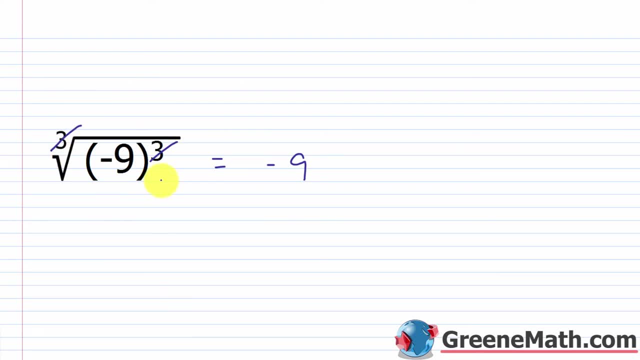 when the index is odd, I can just basically cancel these. When the index is even, I want to cancel them, and then I want to use the absolute value here. So that's the only difference you're watching out for. So now that we've kind of reviewed radicals, let's talk about fractional. 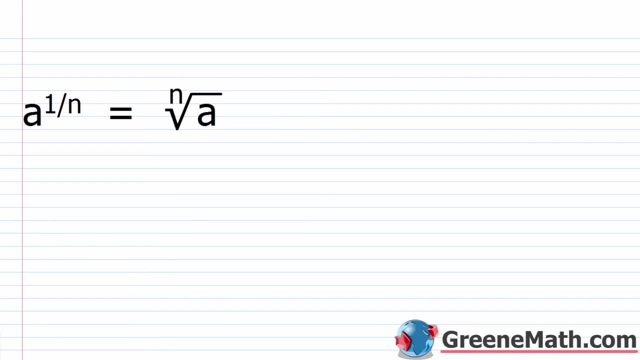 exponents or otherwise called rational exponents. So I want you to recall: if you have something like a raised to the power of 1 over n, this is equal to or the same as the nth root of a. So as an example, let's say I had 4 to the power of 1 half. 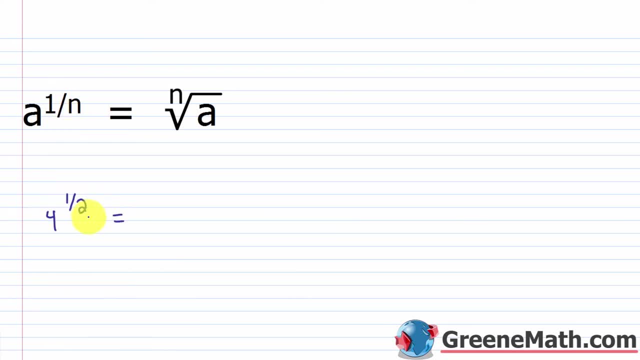 Just kind of following this. what would this be? Well, this part right here becomes your index. So this part right here would be the index. An index of 2 is a square root, So we normally don't display that, but for the purposes here, I'm just going to put a 2 here and then 4, just. 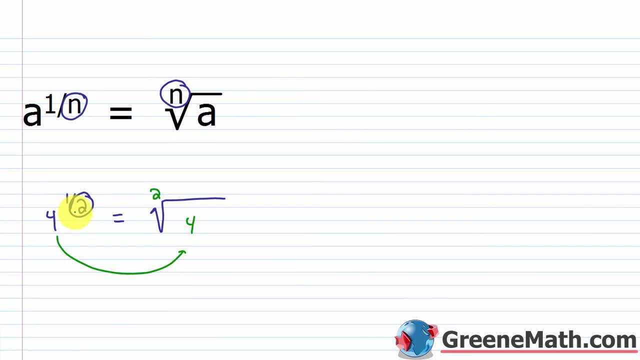 comes over here. So 4 raised to the 1 half power is like taking the square root of 4. And that should make sense because of the rules for exponents. If I have 4 to the power of 1 half and I multiply it by 4 to the power of 1 half, what would that give me? Base stays the same. 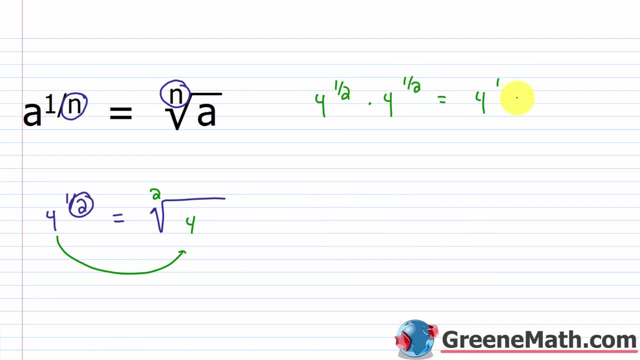 you add your exponents, 1 half plus 1 half is 1.. So this is equal to 4.. If I did this using this and I said, okay, well, this is the square root of 4 times the square root of 4, we would expect. 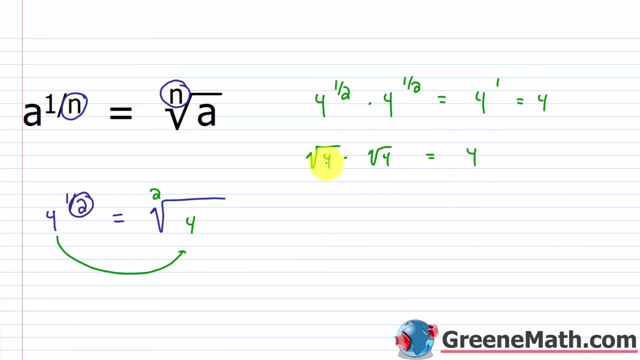 that to be what To be? 4, right, The square root of 4 is 2.. The square root of 4, again, is 2.. 2 times 2 is 4.. So it has to make mathematical sense, and it does. If I wanted something, 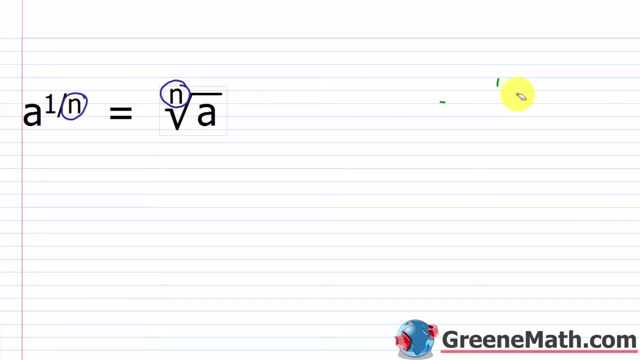 let's say as a cube root. okay, a cube root. So let's say I had 8 to the power of 1 third. Well, this would be the cube root of 8.. Again, whatever's here in the denominator becomes my index or order. 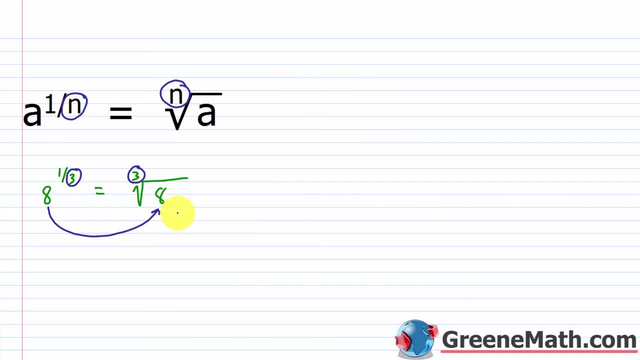 and then it just becomes my radicand. So the cube root of 8 is the same as writing 8 to the 1 third power. Or you can take something way more advanced. Let's say we had, I don't know, 620. 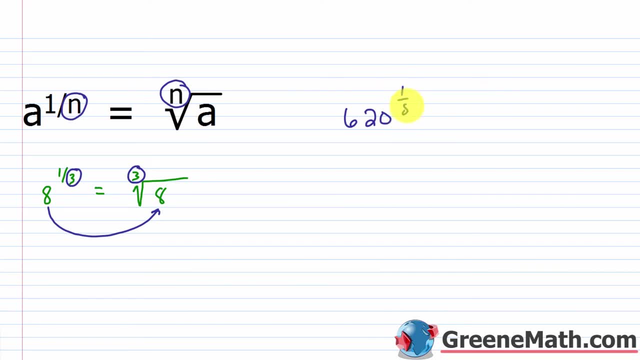 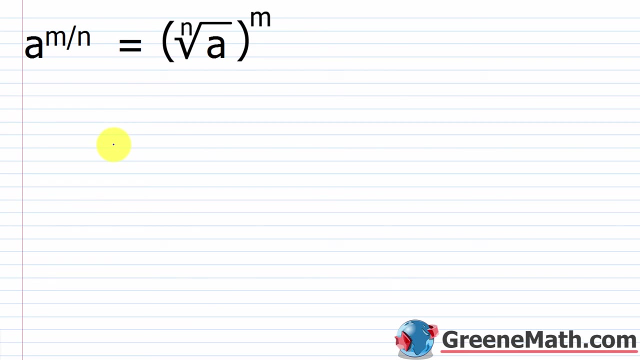 and let's just raise this to the power of 1 eighth as an example. Well, this is what. This is the eighth root of 620, because this part right here goes here and this part right here goes here. So the other thing we need to know with this, let's say we have a raised to the power of m. 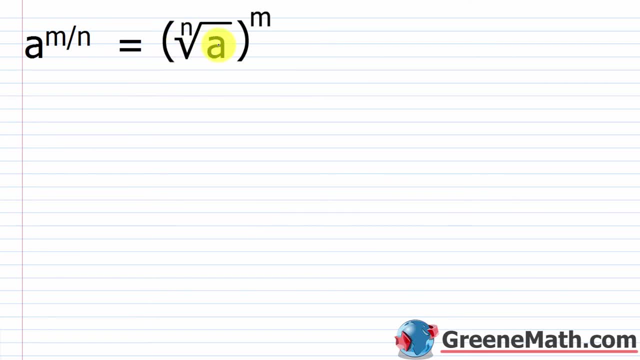 over n. This just gets split up into the nth root of a and this is raised to the power of m. So a good example of this would be something like 9 to the power of, let's say, 3 halves. So just following this, what would you see? Again, the denominator becomes the index. 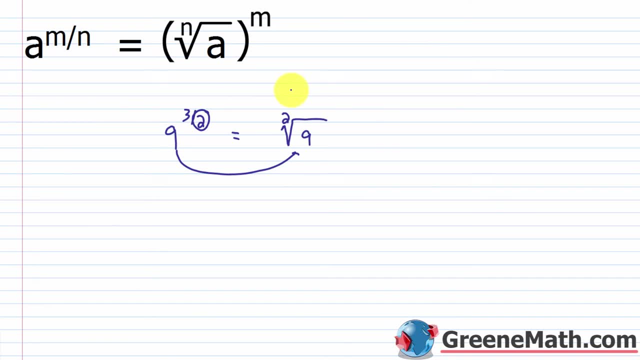 This becomes the radicand, And then this: right here we're going to raise everything to that power. So if I took the square root of 9,, I would get what I would get 3.. And then if I cubed 3,, 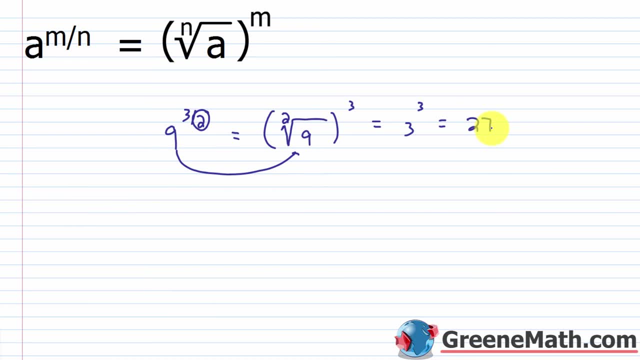 I get what: 3 times 3 is 9.. 9 times 3 is 27.. Now there's other ways to do that. You might see your book tell you to take this guy and raise it to the third power. 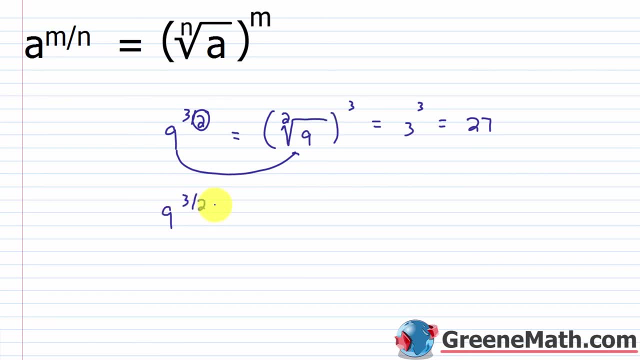 First. so I could also say that 9 to the 3 halves power is what It's: 9 cubed. Okay. so 9 is raised to that power And then we take the square root of that. But this produces a. 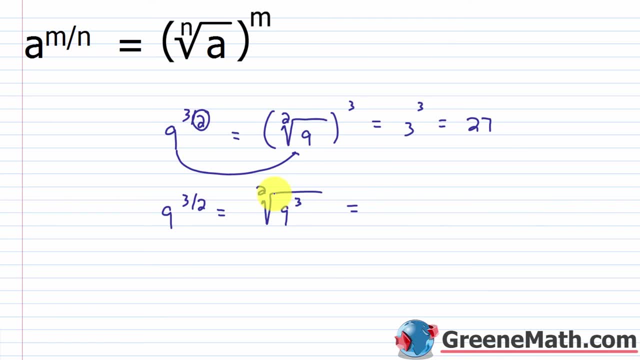 bigger number to take a square root of, And so it's not usually what you want to do. 9 cubed is 729.. So it'd be the square root of 729, which is going to give you 27.. All right, so let's just. 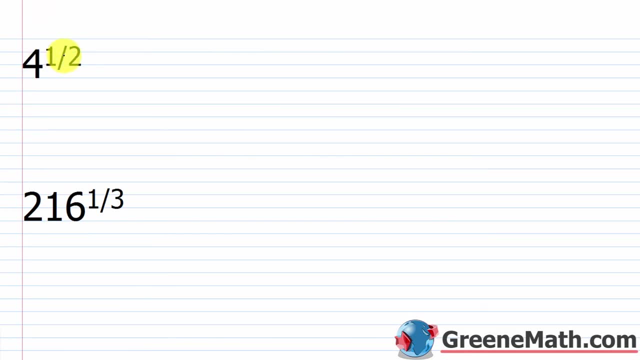 look at some examples. We have 4 to the power of 1 half. We know that's just what. You raise something to the power of 1 half. You're just asking for the square root, So it's the square root of 4.. Now again, you take this right here. that's in. 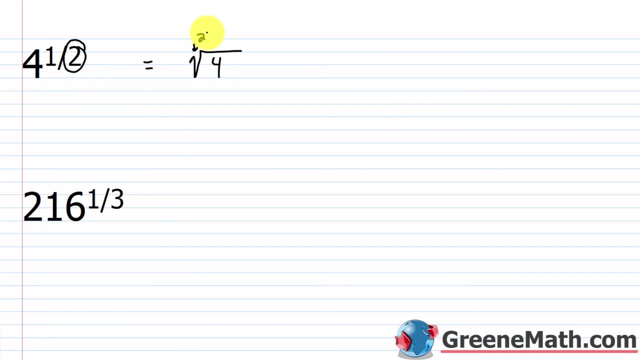 the denominator. That's your index. So the index would be a 2. On a square root. we just don't show that. This right here, this 4, that number, that's the base when we're talking about an exponent. 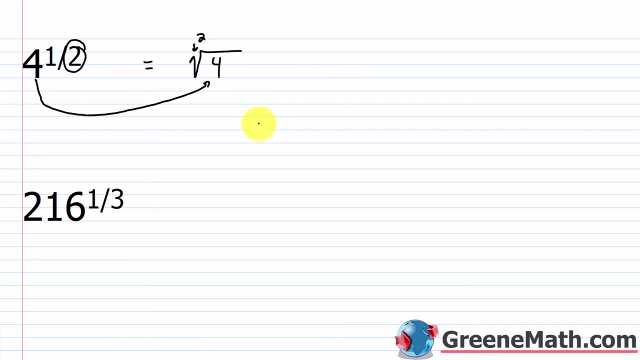 becomes the radicand. So you basically get the square root, or the principal square root of 4, which is 2.. If you look at 216, to the power of 1, third asking for the cube root of 216.. Again, this denominator here becomes the index. 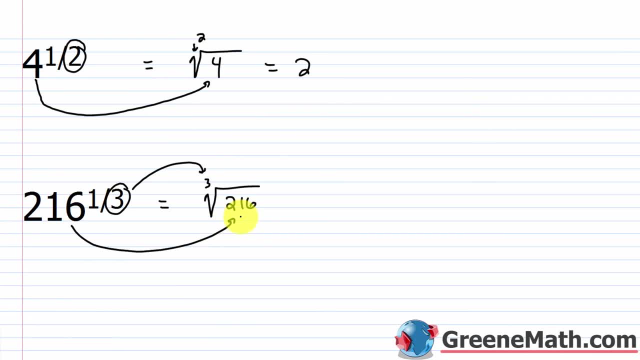 216 becomes the radicand. So what is the cube root of 216?? So if you don't know that off the top of your head, just look at the last two digits: It's a 16.. So you know this is divisible by 4.. So this would be 54 times 4.. 4 is, of course. 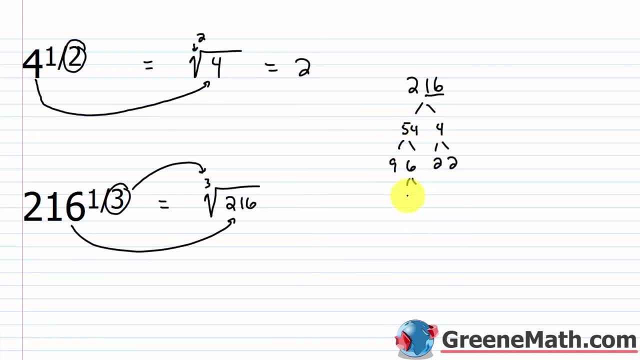 2 times 2.. 54 is 9 times 6.. 6 is 3 times 2 minus 3 times 3.. Now, what do I have here? I have 1, 2, 3 factors of 3 and 1, 2, 3 factors of 2.. 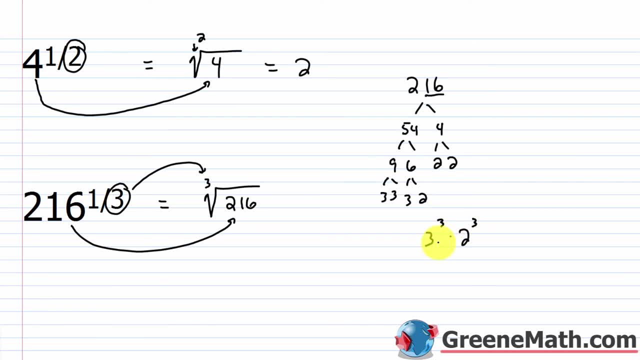 So we've got 3 cubed times 2 cubed. Basically, 3 times 2 is 6.. So it's 6 cubed. So this is equal to what? It's equal to 6, because 6 cubed would give me 216.. So let's take a look at a harder. 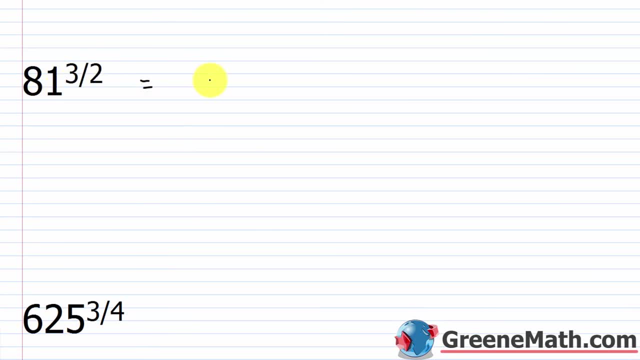 example. So we have 81 to the power of 3 halves. 81 is going to be my radicand. My index is going to be what It's going to be, a 2. So we have 81 to the power of 3 halves. 81 is going to be my. 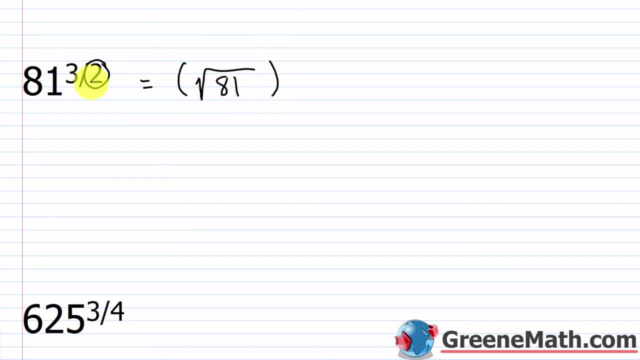 denominator. It's always the denominator, And then I'm raising this whole thing to the power of 3.. So the square root of 81 is 9.. 9 cubed, as we just found out, was 729.. All right, let's take 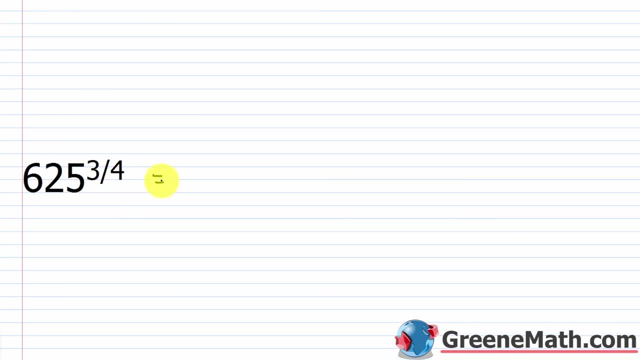 a look at 625 to the power of 3 fourths. So again, 625 is my radicand And the index. here is what It's, a 4.. And then we want this all raised to the third power. So what is the fourth root of 625?? 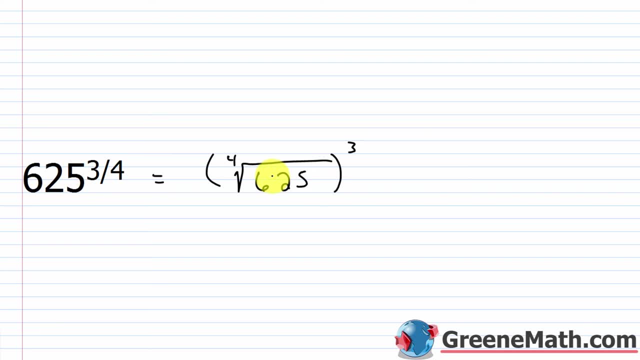 Most of you know that is 5.. 5 times 5 is 25.. 25 times 5 is 125.. 125 times 5 is 625.. So if this becomes 5, when I cube that, I go back to what I go back to 125.. What about if we mix some things? 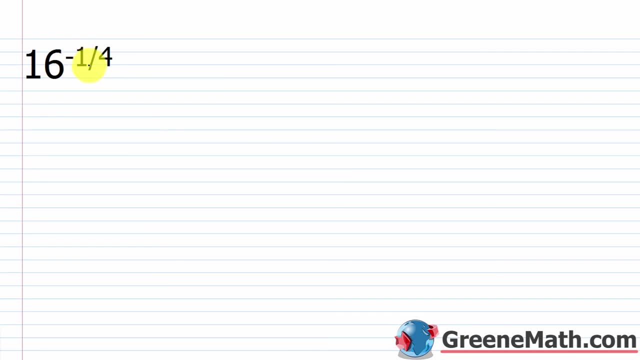 up and we ask for 16 to the power of negative 1 fourth. So what am I asking for here? Well, again, I want the fourth root, I want the fourth root of 16.. And then I would raise everything here to the power of negative 1.. So I can go ahead and take this first. Well, 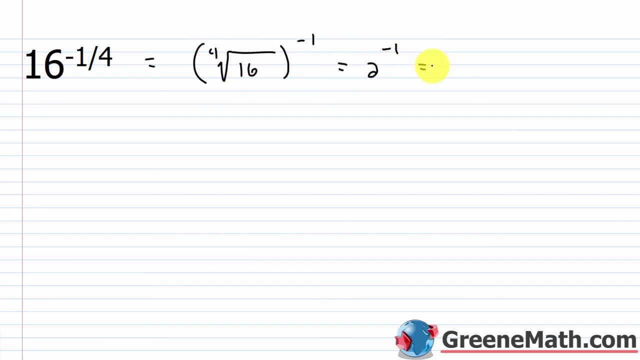 this is 2.. So this would be 2 to the power of negative 1, which is what It's just take the reciprocal of the base, So 1 over 2.. Raise this to a positive 1, which is basically just 1 half. 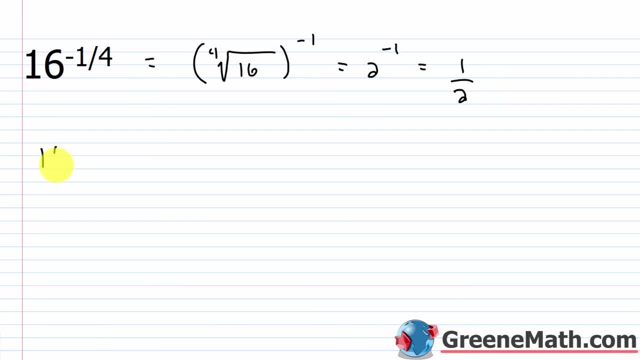 Now the other way to do this. if you wanted to, you could say: OK, I have 16 to the power of negative 1 fourth. Well, you could have started out by saying: I have 16 raised to the power of. 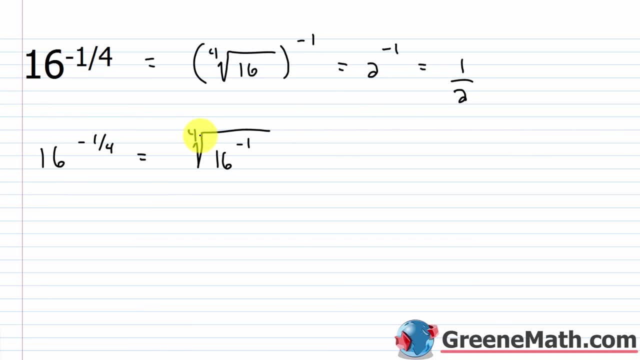 negative 1.. And then I'm going to take the fourth root of that Same answer. either way, This would be what. This would be the fourth root of take the reciprocal of this. This is 1 over 16.. And it's a little bit more complex here because it's a fraction, But just think about the fourth root. 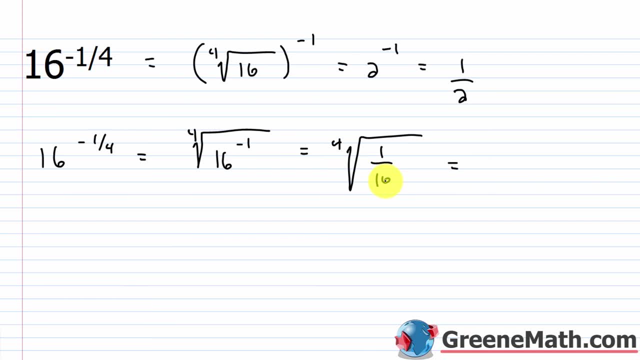 of 1 over 16.. Well, 1 half times 1 half times 1 half times 1 half is going to give you 116.. You know, 1 to the fourth power is 1.. So that's easy. And then what to the fourth power of 16? Well, 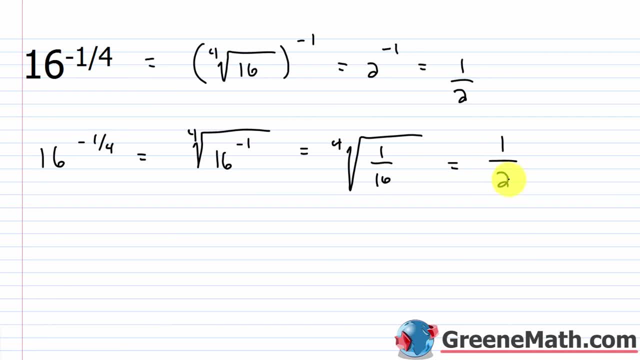 that's 2.. So you end up with 1 half either way. Now what about something like negative 32 to the three fifths power? Well, again we're looking at we have negative 32.. And then I'm going to. 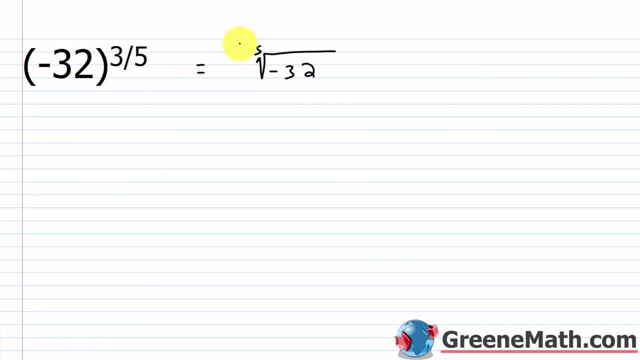 take the fifth root of that And I'm going to raise the whole thing to the third power. So what's the fifth root of negative 32? That's going to give us negative 2.. And we want to cube that Negative 2. cubed is negative 8.. But the next one, we're going to look. 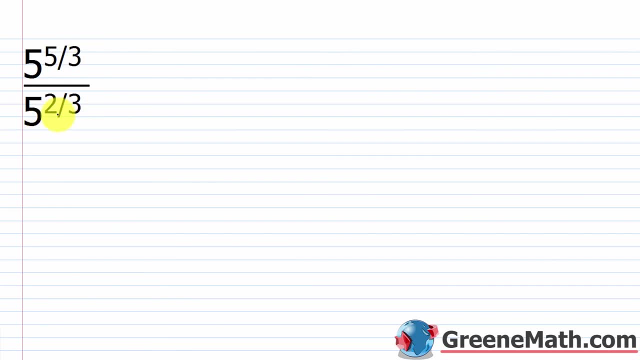 at is 5 raised to the power of 5 thirds over 5 raised to the power of 2 thirds. Now, just as we saw when we worked with exponents in the past, if you have the same base, which we have, a base of, 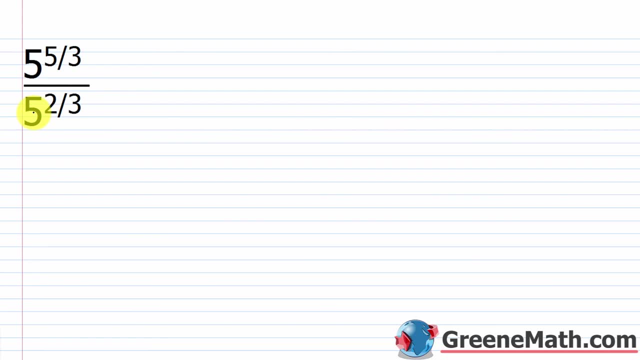 5, a base of 5, and you're dividing. you subtract the exponent in the numerator minus the exponent in the denominator, So 5 just stays the same And we would do 5 thirds minus 2 thirds. Same rules apply No matter what you're working on, no matter how complex it is. 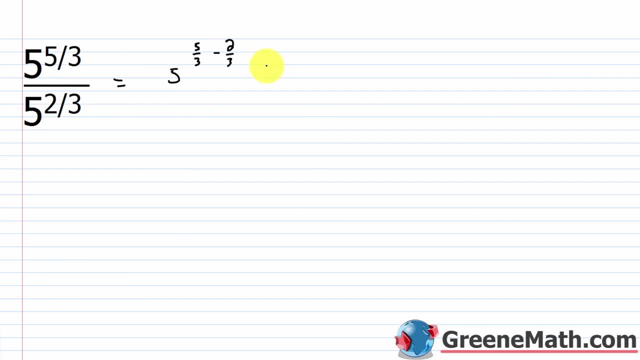 you always go back to those basic rules that you learned. So 5 minus 2 is what That's, 3.. So you would have 5 raised to the power of 3 over 3, which is 5 to the power of 1.. It's just 5.. 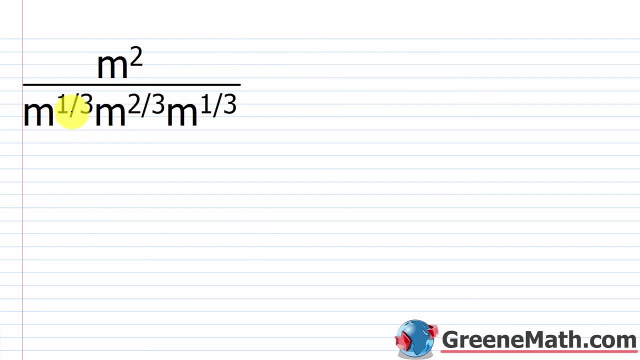 All right, say we take a look at m squared over, m to the power of 1 third times m to the power of 2 thirds times m to the power of 1 third. So again, same rules apply. So m squared, squared over. I'm just going to use my product rule for exponents: m would stay the same. 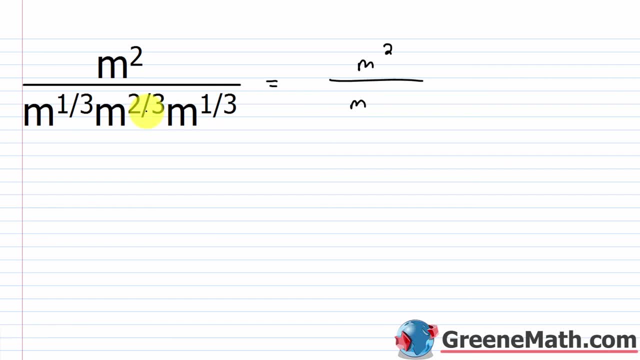 And we would add all these exponents. So we know that 1 third plus 2 thirds is 3 thirds. 3 thirds plus 1 third is 4 thirds. So what would happen here is, if I'm dividing, m stays the same And we would do 2,- which is the exponent in the numerator- minus 4 thirds. 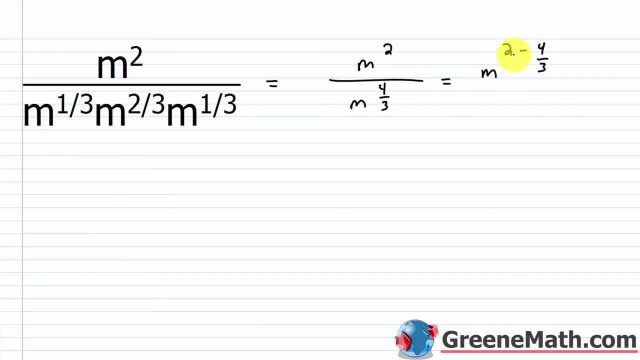 which is the exponent in the denominator. To get a common denominator, I would write 2 as what 6 thirds, And we'd end up with m to the power of 6 minus 4 is 2, and then over 3.. 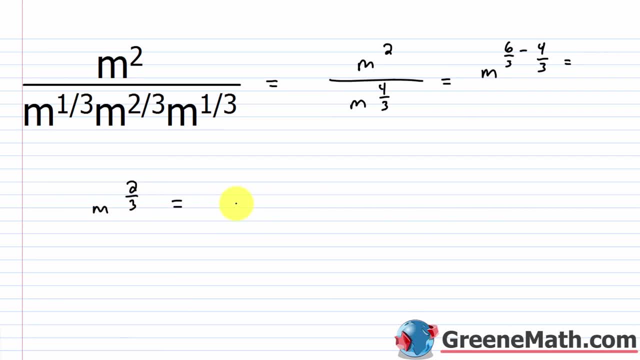 So you can leave it in this format, or you could write that you have the cube root of m, That's squared. Or you could say you have m squared and take the cube root of that. All of these are the same. What about m? cubed squared times, m squared over m to the power of 1? 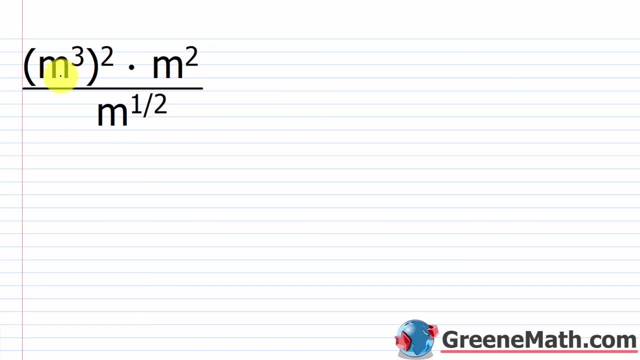 half m squared over m to the power of 1 half. So you could write that you have the cube root of m to the power of 1 half. Well, using my power to power rule here, I know this would be m to the 6th power. 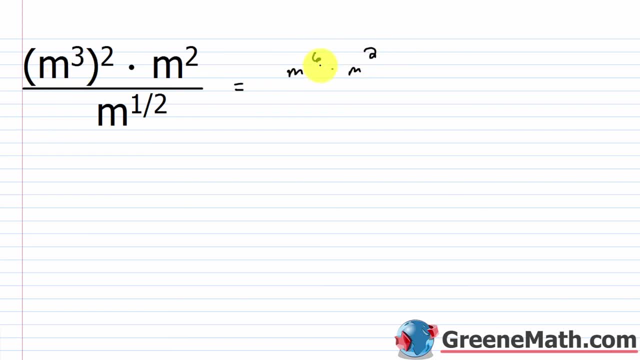 and times m squared. All I would do is add exponents here. So m would say the same: 6 plus 2 is 8.. So this would basically be m to the 8th power over m to the power of 1 half. 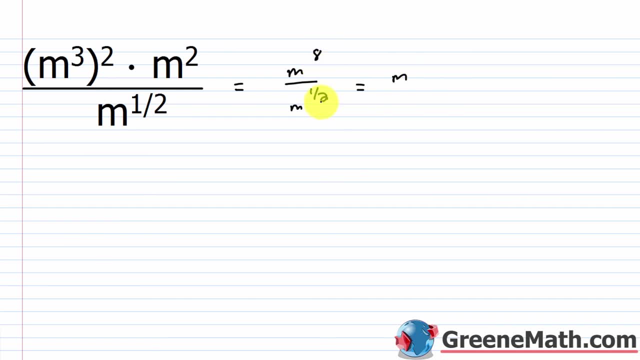 So m stays the same And I would take 8, and I would subtract away a half. So let's write this as 16 over 2 minus 1 over 2. This would equal m to the power of 1 half. 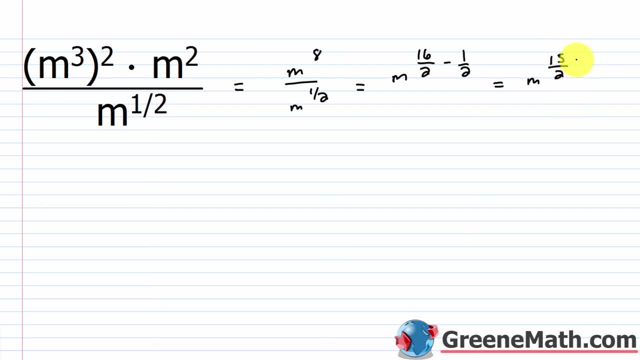 15 over 2.. Again, you could leave it like that, or you could write that you have the square root of m raised to the 15th power, Or you could say you have m to the 15th power, and then you could. 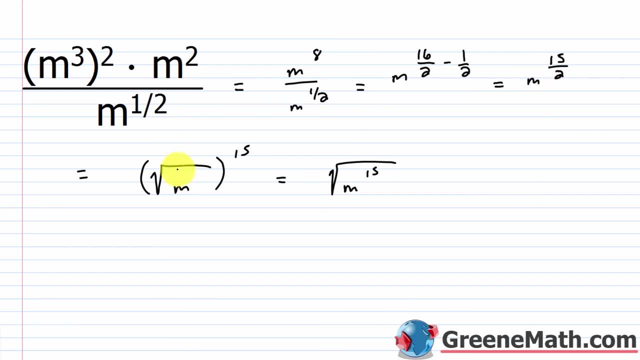 take the square root of that. All of these, this one, this one and this one mean the exact same thing. All right for the last one. we have x squared raised to the 2, 3rd power times: x to the. 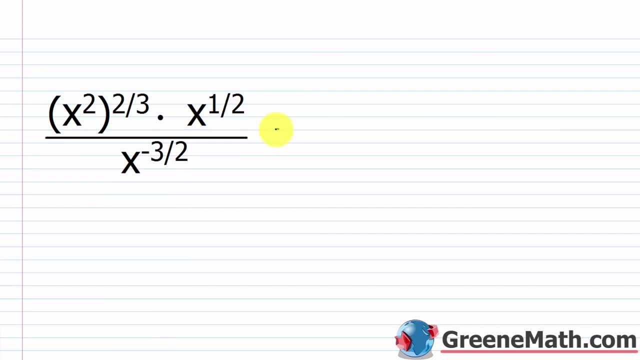 power of 1 half over x to the power of negative 3 halves. So if I look at this, I use my power to power rule. I would multiply 2 times 2 and get 4.. So this would be x to the power of 4 3rds. 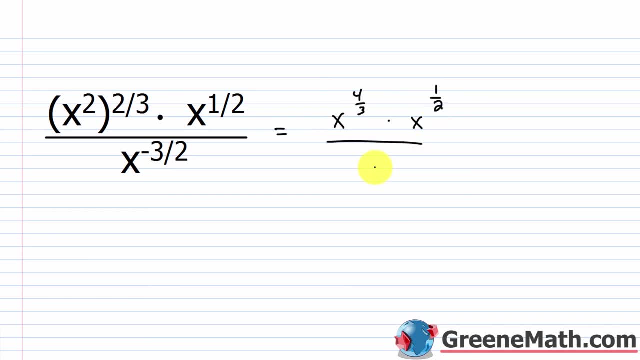 And then we multiply by x to the power of 1 half, And of course this is over x to the power of negative 3 halves. So let's put this as equal to. let's deal with the numerator first. So we have: 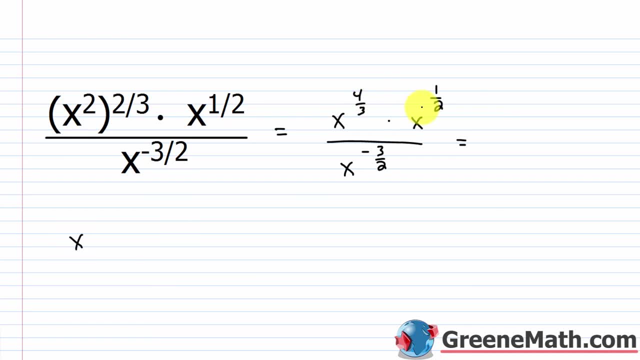 what We have, x staying the same and we're going to add the exponents. So if I add 4 3rds plus 1 half, multiply this by 3 over 3, multiply this by 2 over 2.. 2 times 4 is 8.. So you're going to have 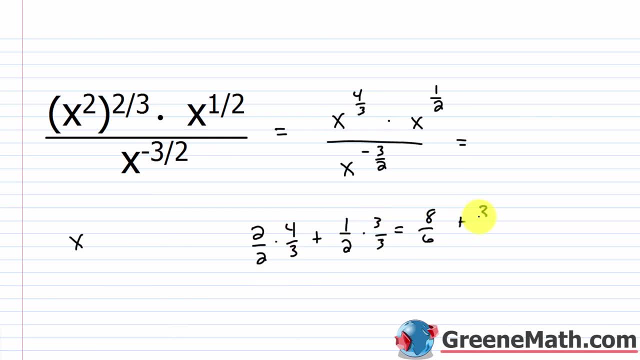 what You'd have. 8 over 6 plus 1 over 3 is 3 over 6.. 8 plus 3 is 11.. So this would be x to the power of 11 sixths. Then this is over x to the power of negative 3 halves. Now I don't need to. 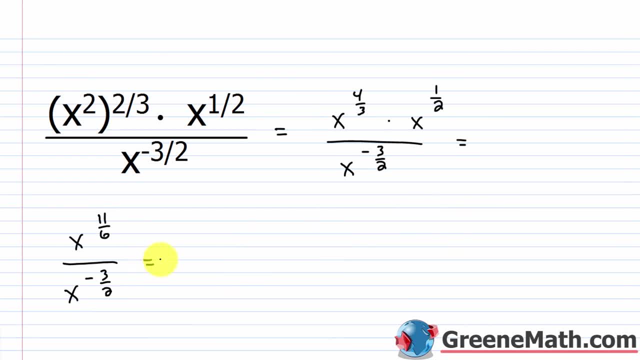 do anything fancy here other than leave x the same and then just subtract. So I would do 11 sixths minus a negative. Notice that that's a negative and I'm subtracting it away. So that's plus a positive, So that's negative. 3 halves. So to get a common denominator, let's multiply this by 3 over 3.. And